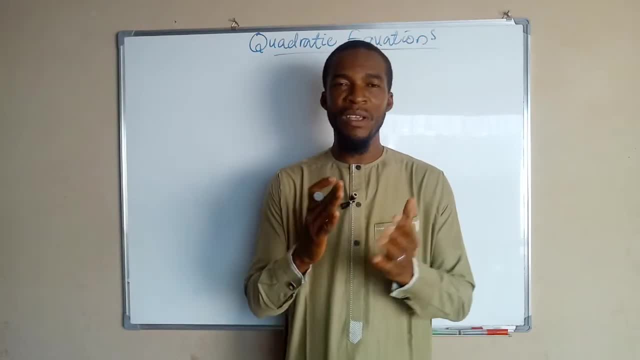 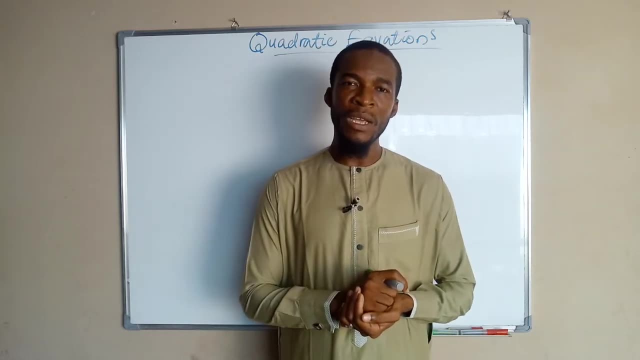 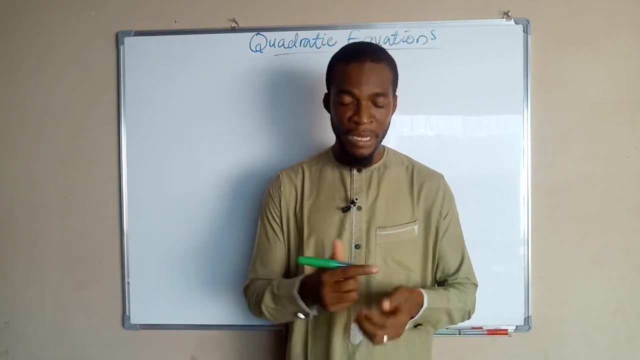 In today's tutorial I'm going to tell you most of the things you need to know about quadratic equation and how to solve quadratic equation via factorization. So if you're new here, consider subscribing. press the bell icon so that you will be notified whenever I uploaded new content. Basically, the 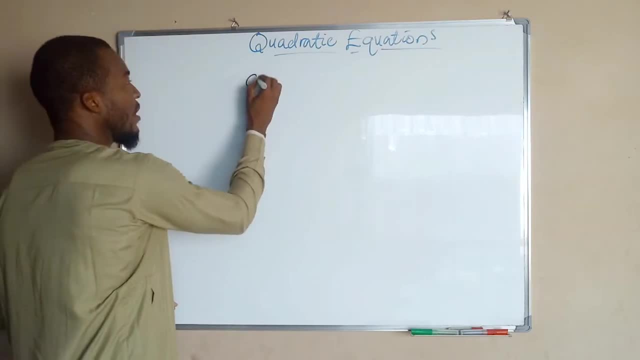 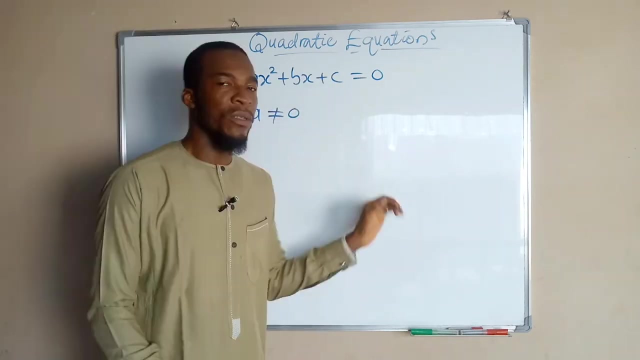 general form of a quadratic equation is written as: ax squared plus bx plus c equals 0, for which a is never equal to 0 but b and c can be equal to 0. So we say a quadratic equation is a polynomial equation of degree 2.. The highest degree. 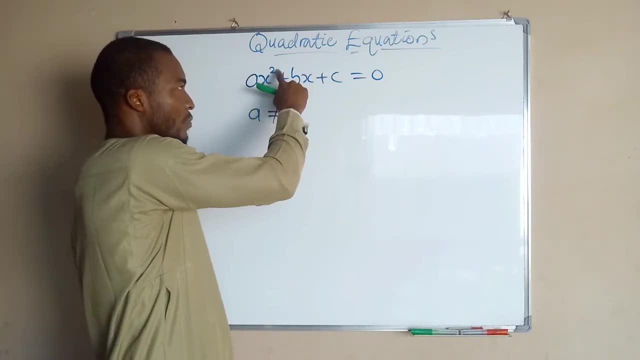 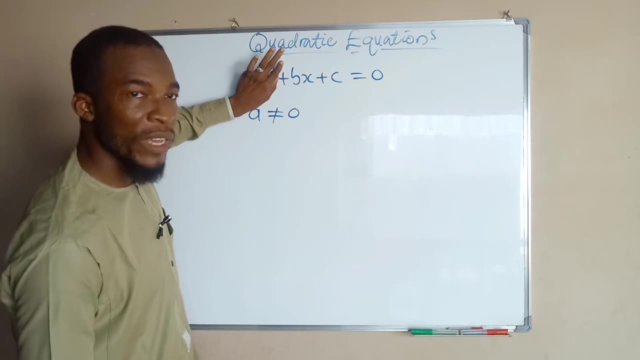 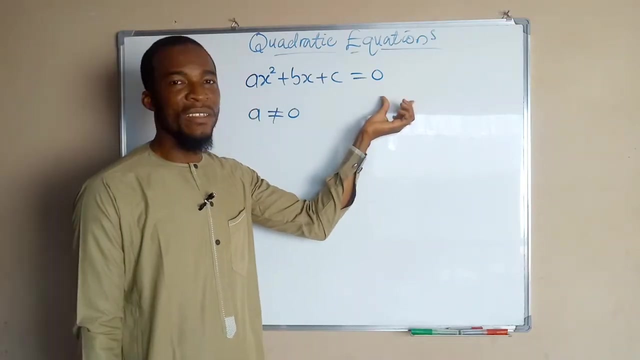 for a quadratic equation is 2.. Why a is never equal to 0 is is because if a equal to 0, the whole of this term will vanish, leaving a linear equation. So why do we always have 0 to the right hand side? It is not necessary that we 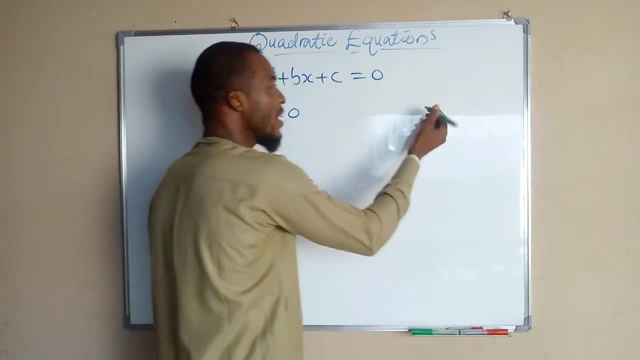 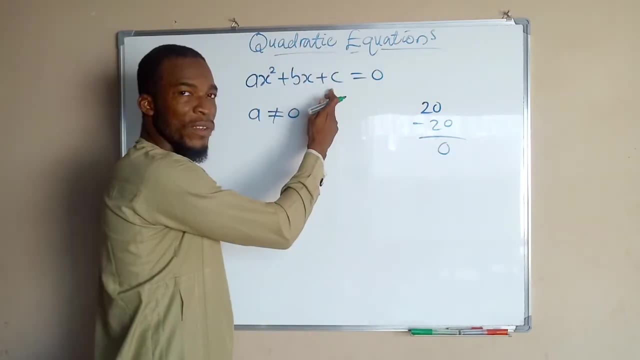 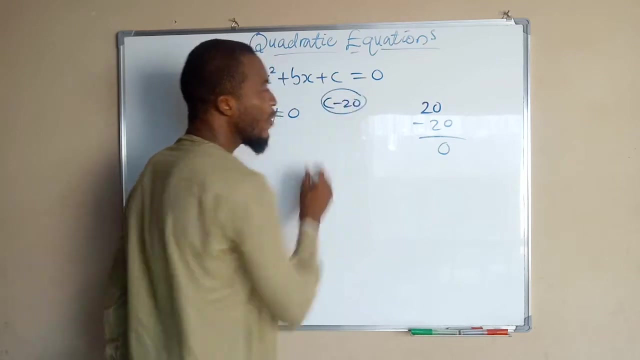 must have 0, but no matter what number is here, say 20.. Once you subtract 20 from that side, you'll be left with 0, and we have another constant here which we have to subtract 20 from. So we have c minus 20 and the whole of this remains. 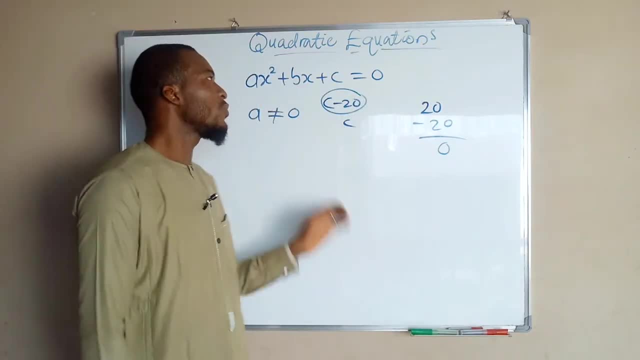 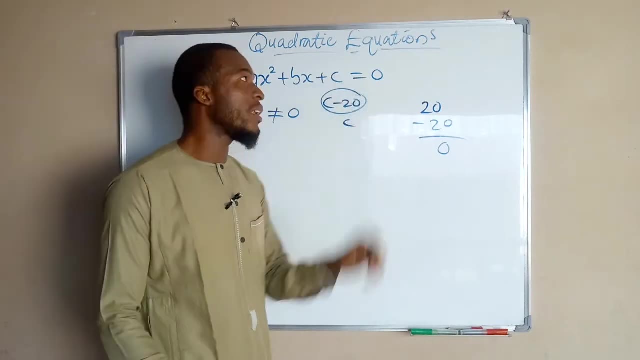 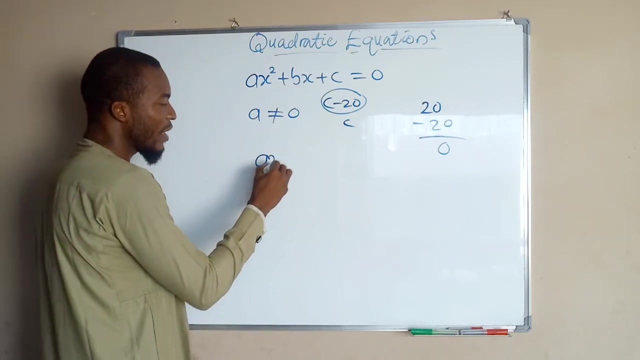 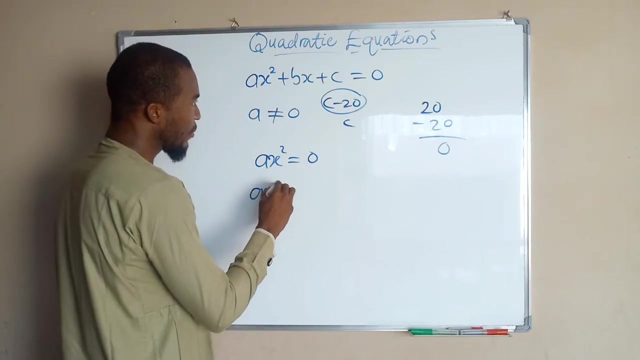 constant which can be written as c, So we call it quadratic, because the highest degree is 2 and it is an equation because of the equality sign, Since b and c can appear to be equal to 0. we may have a quadratic equation in the form of ax squared equal to 0.. We may have ax squared plus bx, equal to 0. 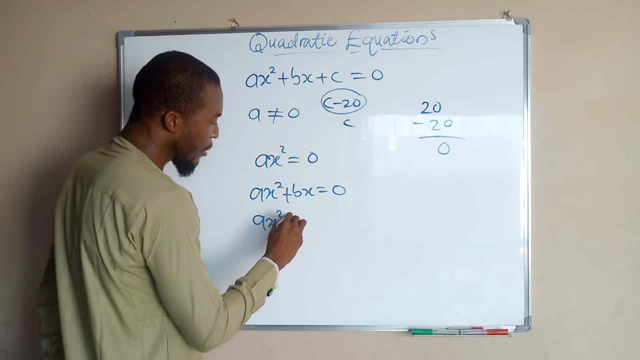 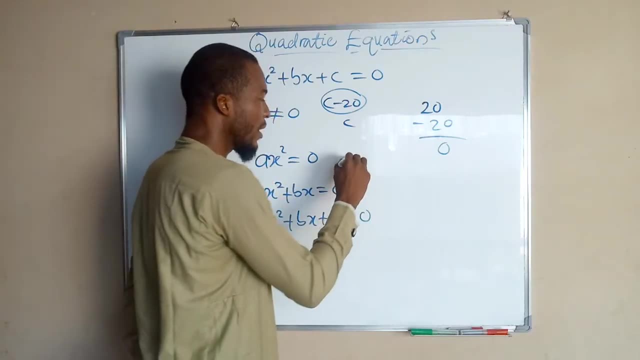 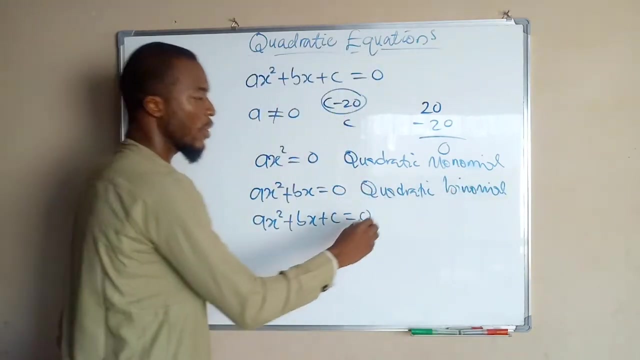 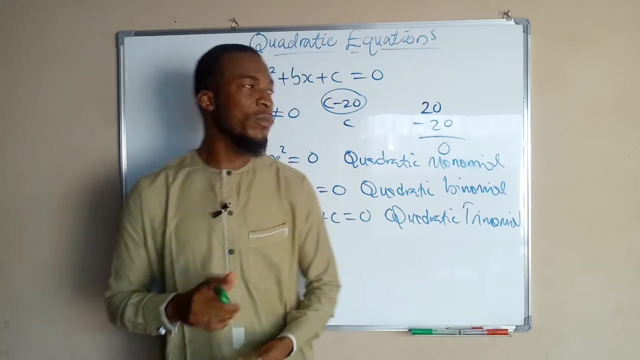 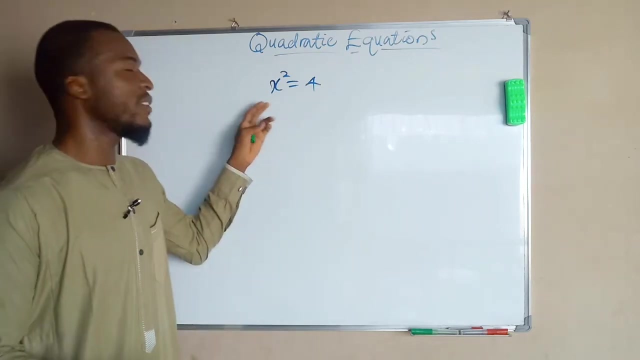 or we may have ax squared plus bx plus c, equal to 0.. So this is called a quadratic monomial, This is a quadratic binomial and this is quadratic trinomial. Now let us see how we can solve quadratic equations by factorization. Suppose we have x squared equals to 4.. We want to solve this. 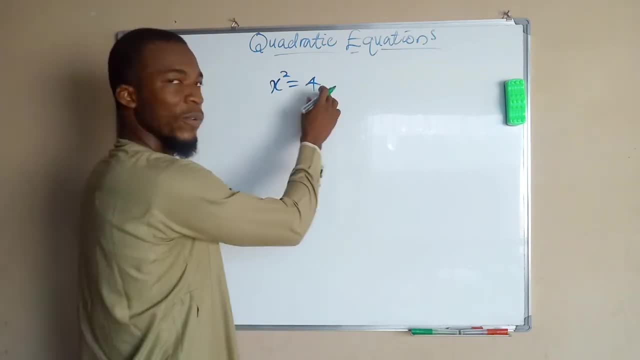 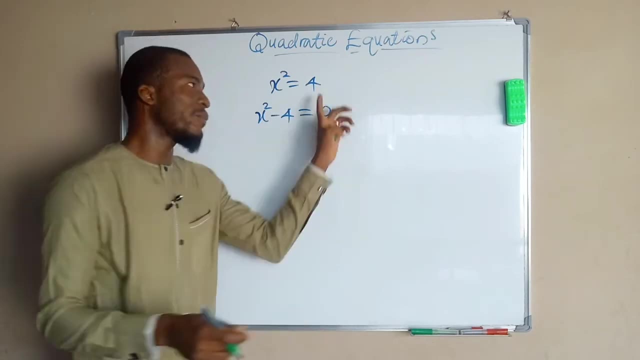 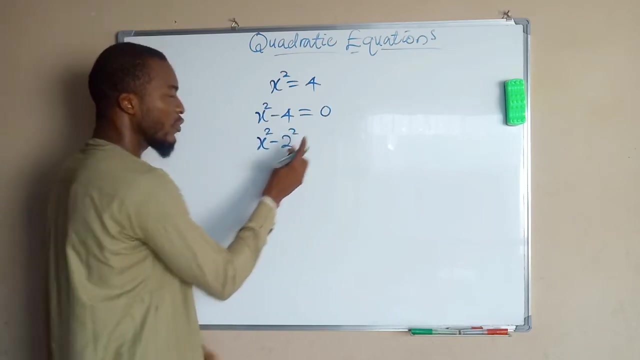 by factorization. You know that we can subtract 4 per inverse side so that we have x squared minus 4, and to the other side we have 0, since we have subtracted 4 from that side. and this can also be written as x squared minus 2, squared because 2. 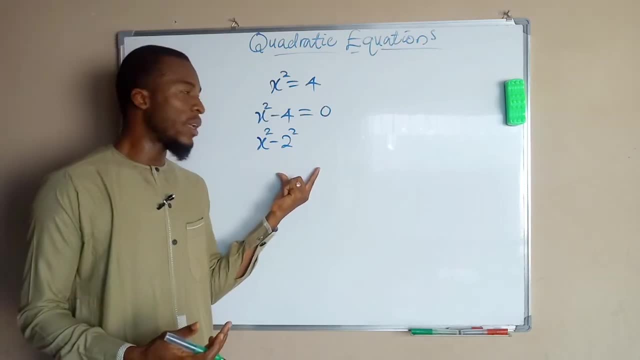 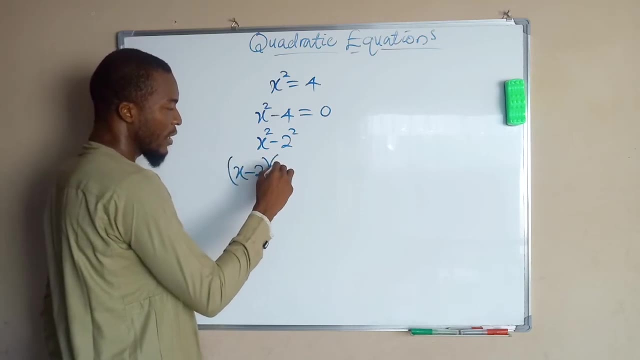 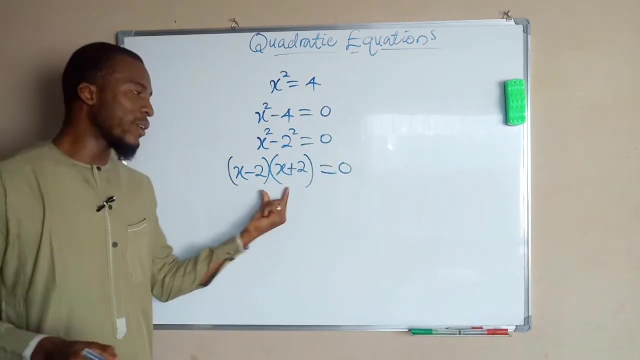 squared is equal to 4, which are difference of 2 squares, and if you have difference of 2 squares you can factorize them as x minus 2, then x plus 2 and the whole of them equal to 0, where we have two factors multiplying each. 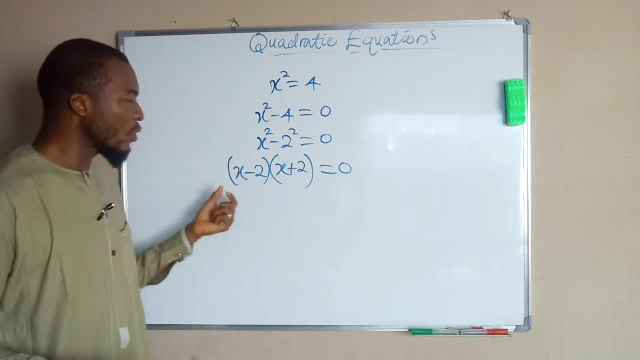 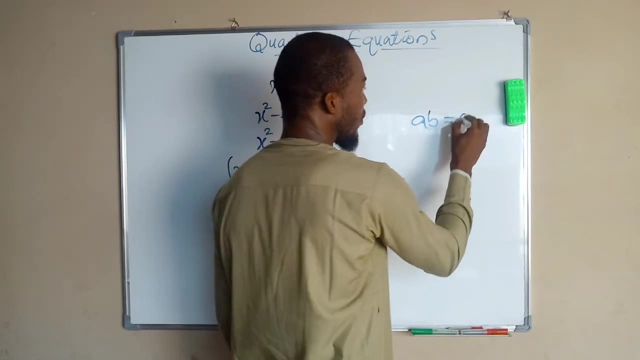 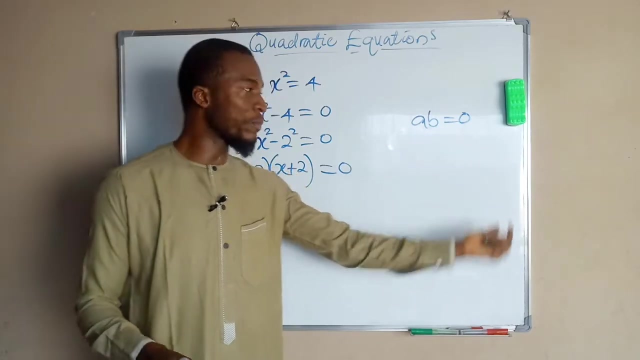 other and the result is 0. so on what condition will you multiply two numbers to get 0? suppose we have a multiplying B and the result is 0. this implies that either a or B is equal to 0. for this equation to be true, because if a is 0, we? 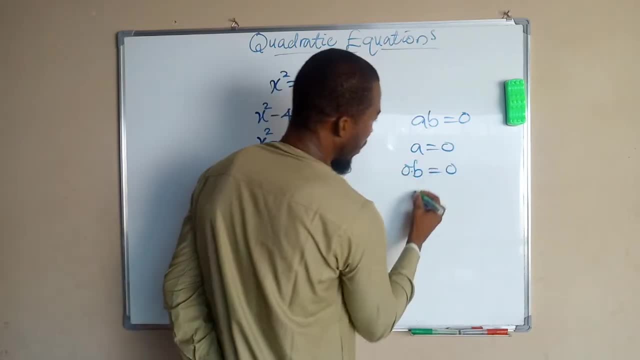 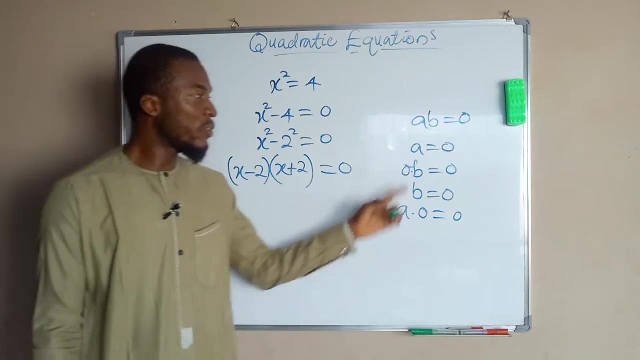 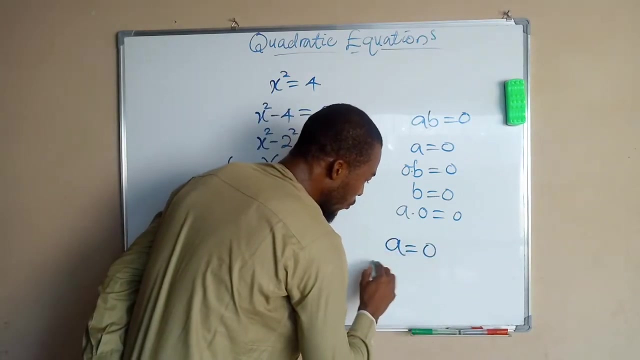 have 0 times B equals 0, and if B is 0, we have a multiplying 0 as equal to 0. but since we don't know among these two factors which one is 0, we may say a can be equal to 0 or B equal to 0. 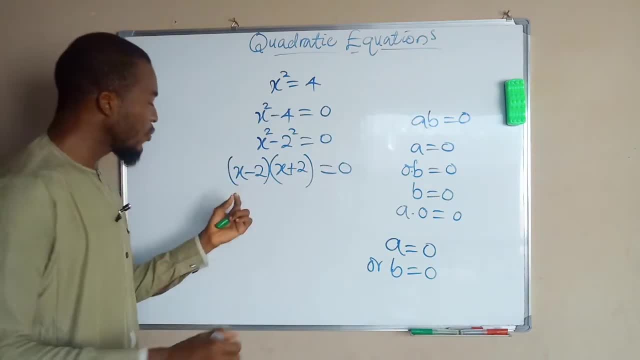 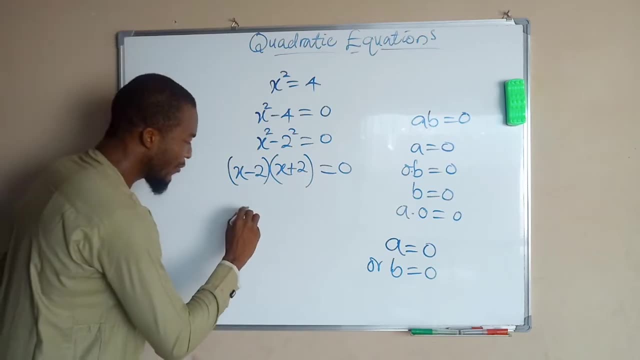 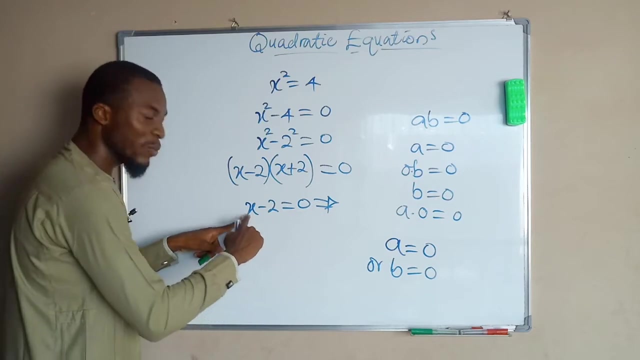 and the same principle is applicable here, since we don't know which among these two factors is 0, so we are going to set each one of them to be equal to 0. if you set x minus 2 equals to 0. this implies that, for this equation to be true, x must be equal to 2. 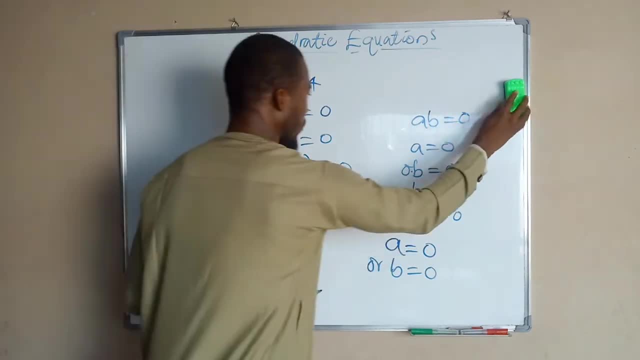 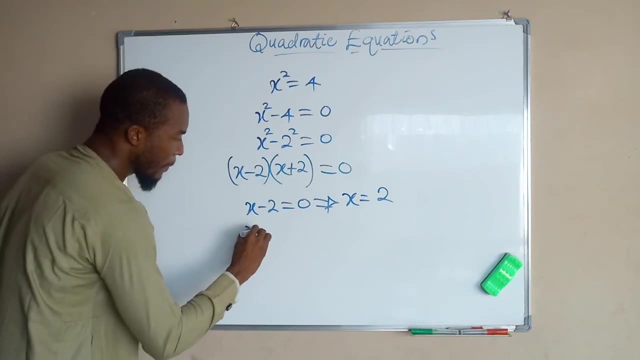 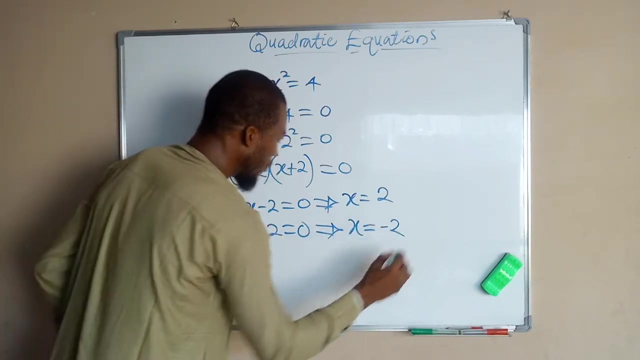 because 2 minus 2 is equal to 0. this implies that x is equal to 2, and for the second one, which is x plus 2 equal to 0, this implies that x must be equal to negative 2 for this equation to be true, because negative 2 plus 2 is 0.. So hence, 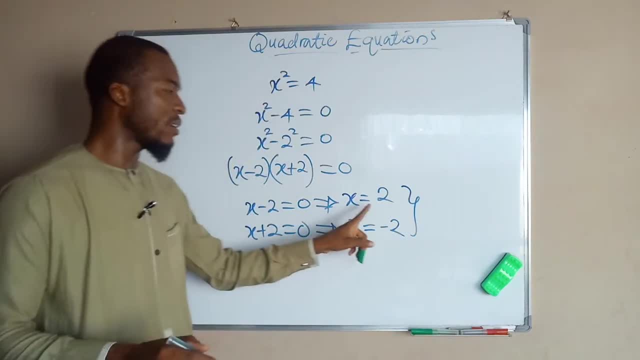 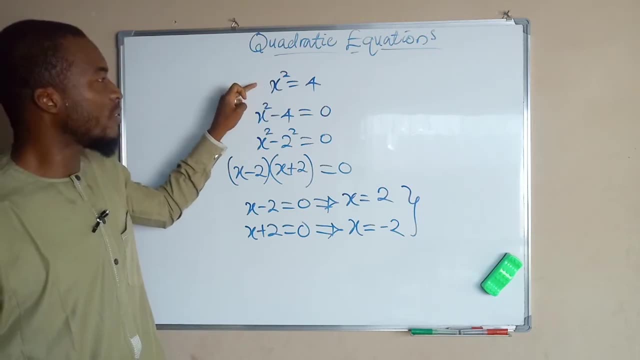 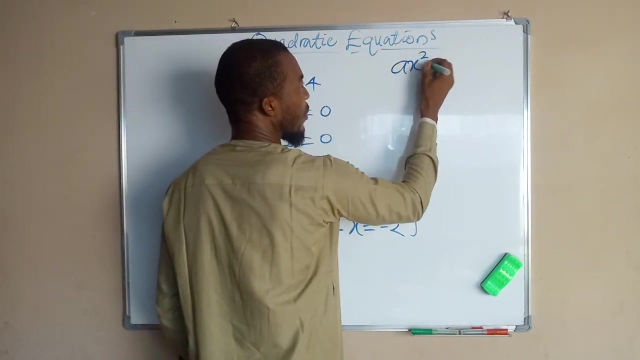 the two real values of this equation are positive 2 and negative 2.. So what about if a is not 1? because, if you can see here, the leading coefficient, which is a, remember the general form- is ax squared plus bx plus c equals to 0.. The 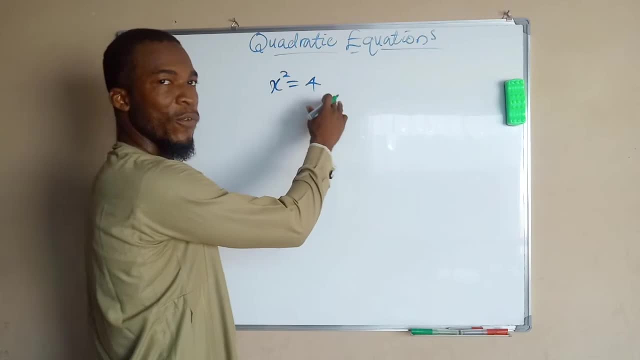 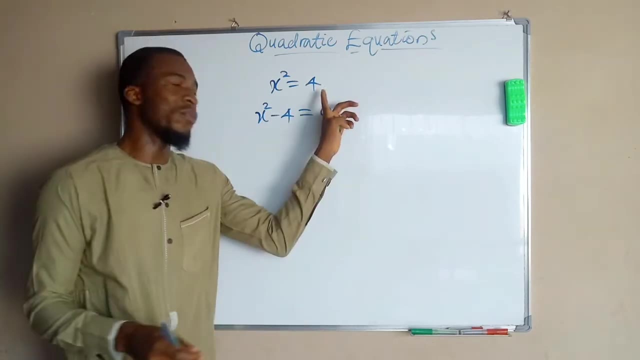 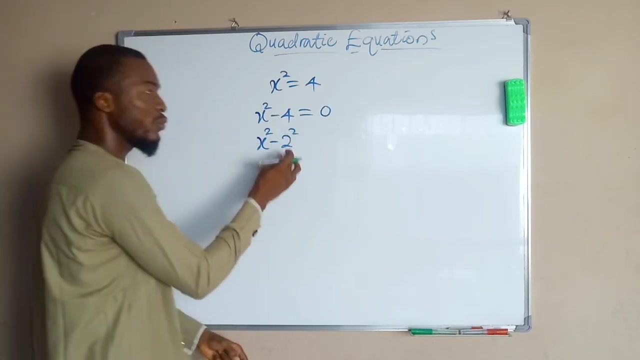 factorization. You know that we can subtract 4 per inverse side so that we have x squared minus 4, and to the other side we have 0, since we have subtracted 4 from that side. and this can also be written as x squared minus 2, squared because 2. 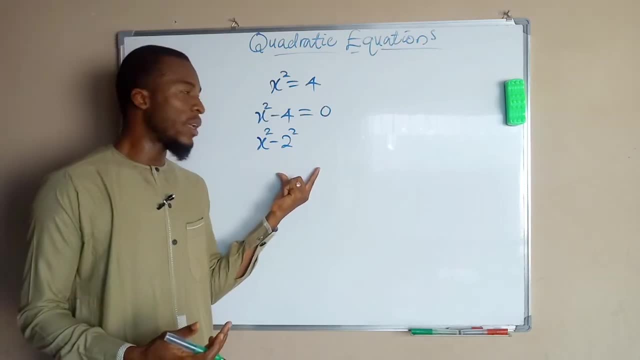 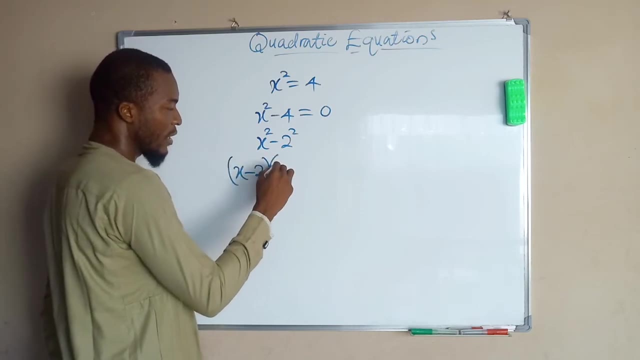 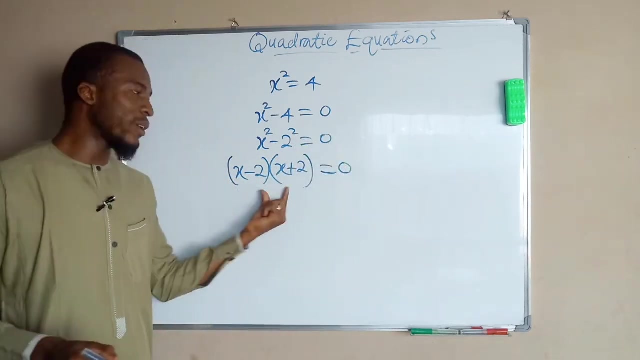 squared is equal to 4, which are difference of 2 squares, and if you have difference of 2 squares you can factorize them as x minus 2, then x plus 2, and all of them equal to 0, where we have two factors multiplying each other. 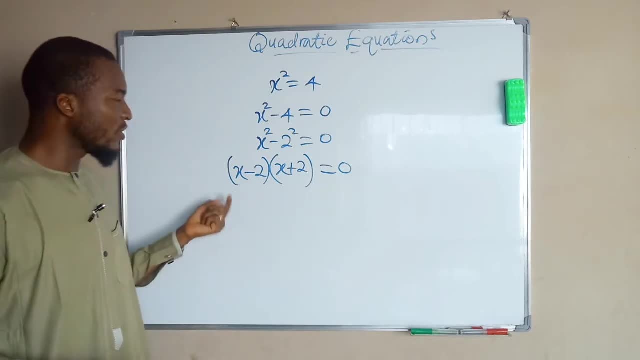 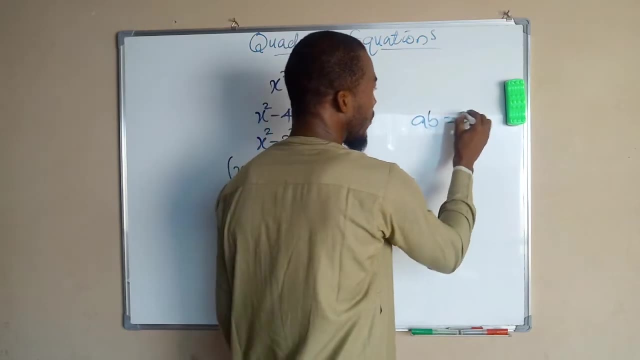 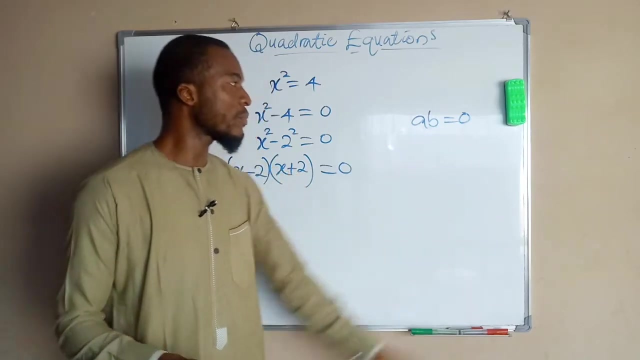 and the result is zero. so in what condition will you multiply two numbers to get 0?? So first we have a multiplying b and the result is 0. this implies that either a or b is equal to 0 for this equation to be true, because if a is 0, 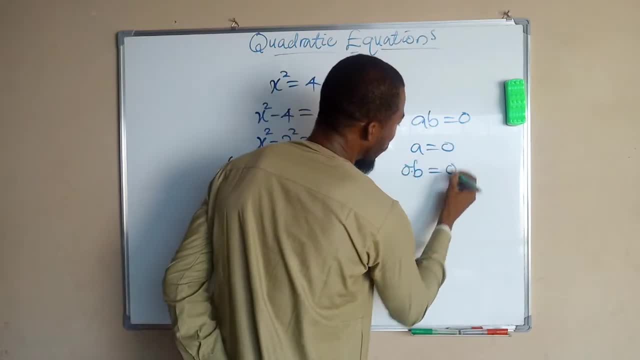 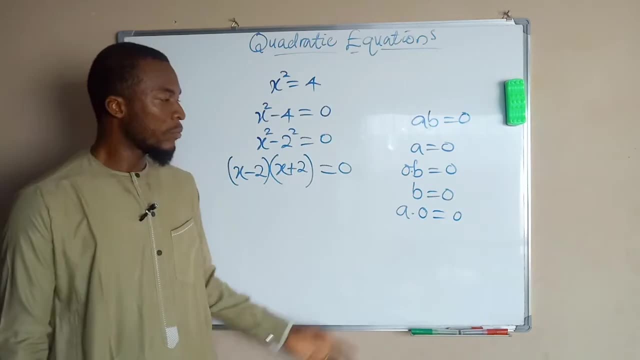 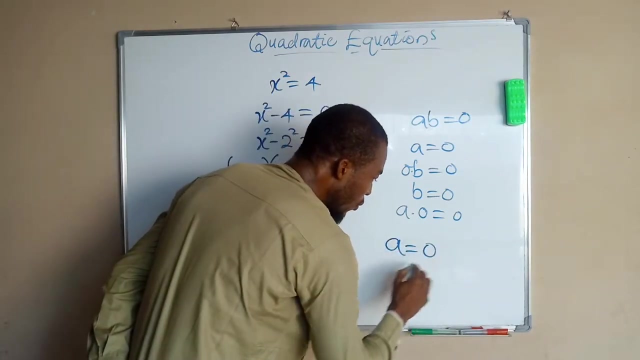 we have 0 times b to 0, and if b is 0, we have a multiplying 0 as equal to 0. but since we don't know among these two factors which one is 0, we may say a can be equal to 0 or b. 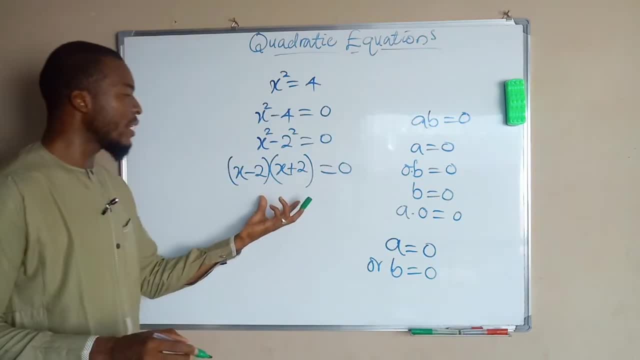 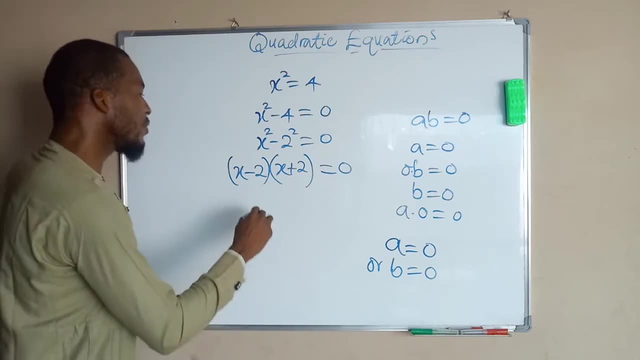 equal to 0, and the same principle is applicable here, since we don't know which among these two factors is 0, so we are going to set each one of them to be equal to 0. if you set X minus 2 equals to 0, this implies that for this: 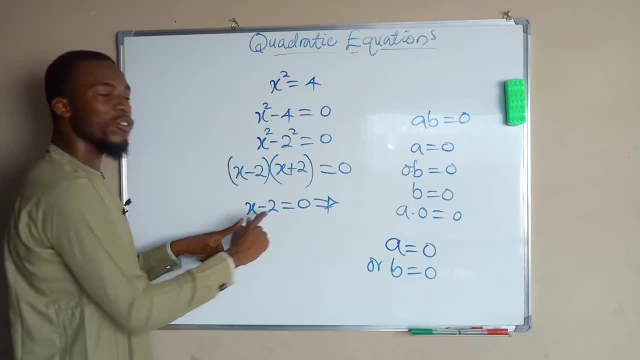 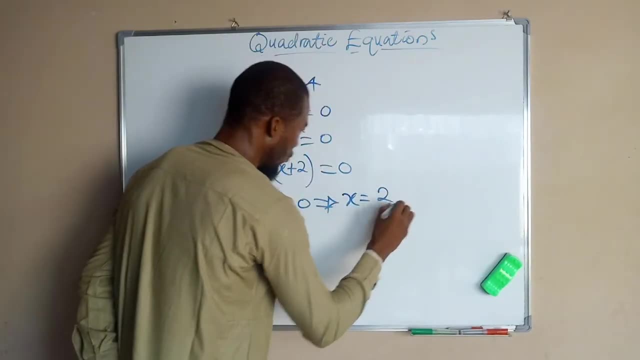 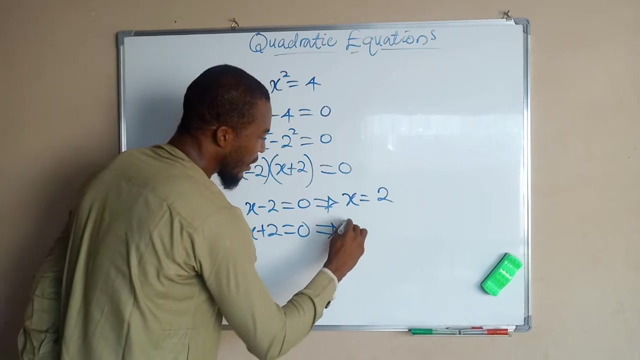 equation to be true, X must be equal to 2, because 2 minus 2 is equal to 0. this implies that X is equal to 2 and for the second one, which is X plus 2, equal to 0. this implies that X must be equal to negative 2 for this equation to be true. 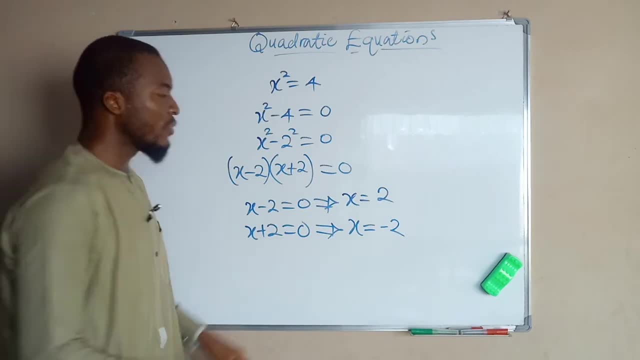 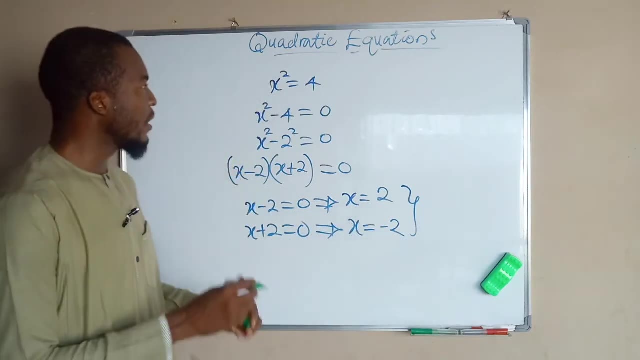 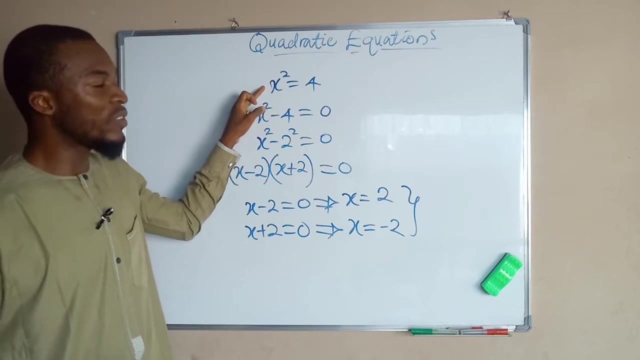 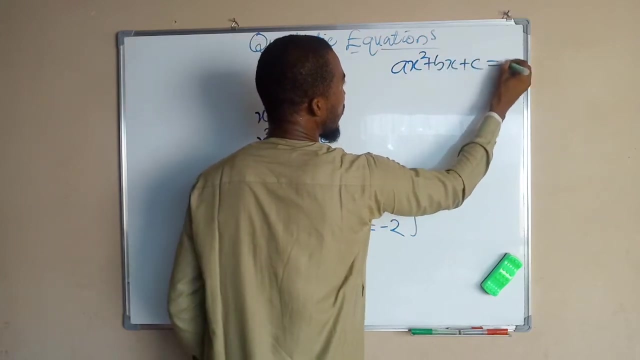 because negative 2 plus 2 equals to 0. so hence the two real values of this equation are positive 2 and negative 2. so what about if A is not 1? because, if you can see here the leading coefficient, which is A, remember the general form is: AX squared plus BX plus C equals to 0. 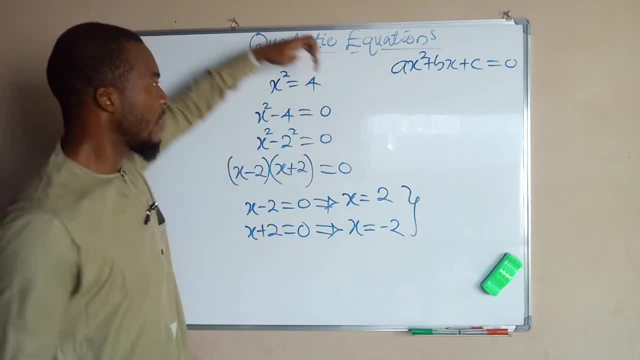 the coefficient of X squared is always A. in this equation you can see that A is equal to 0 and the coefficient of X squared is always A and this equation you can see that A is equal to 0 to 1. this is why we don't have any number attached to x squared. so first, 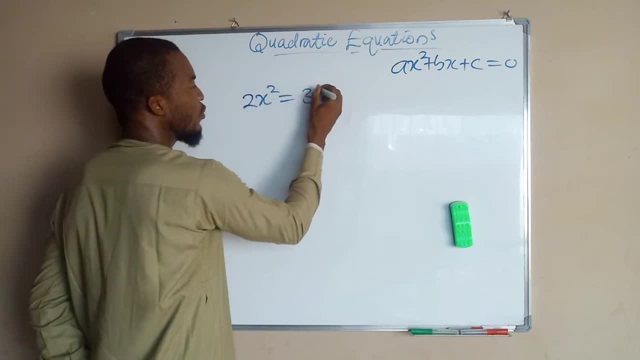 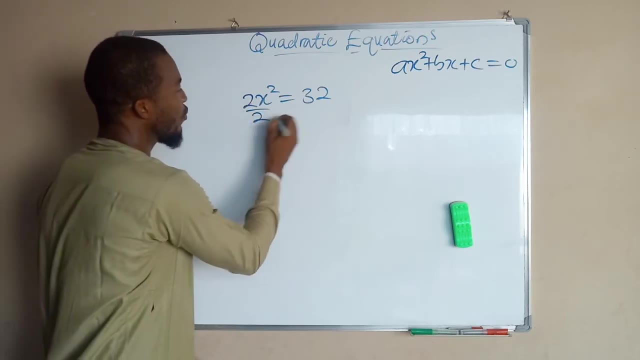 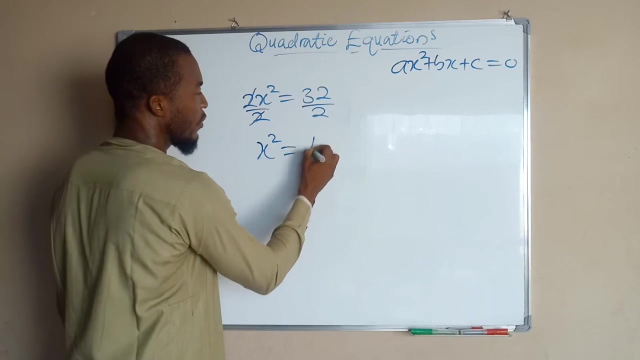 you have 2x squared equals to 32. here the leading coefficient is equal to 2. to get rid of this 2, you can divide both sides by 2. so we do divide both sides by 2, which 2 cancels 2, leaving x squared equals to 16, because 32 divided by 2 is. 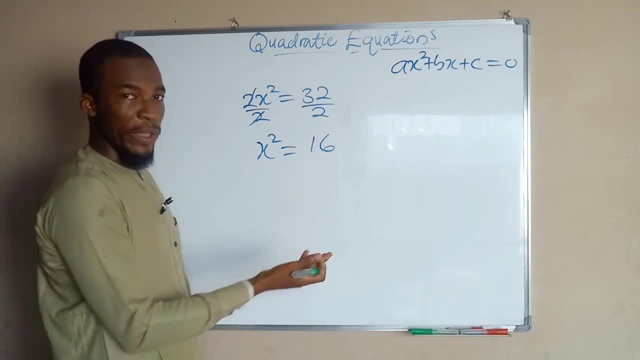 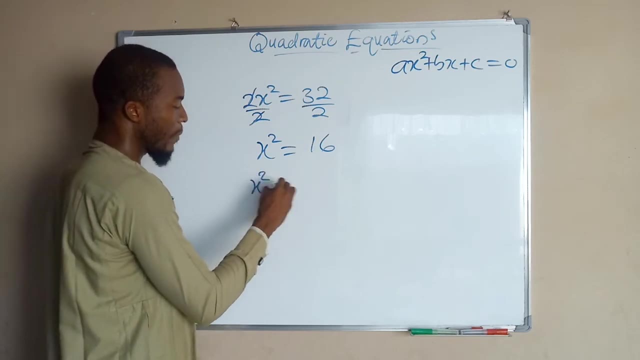 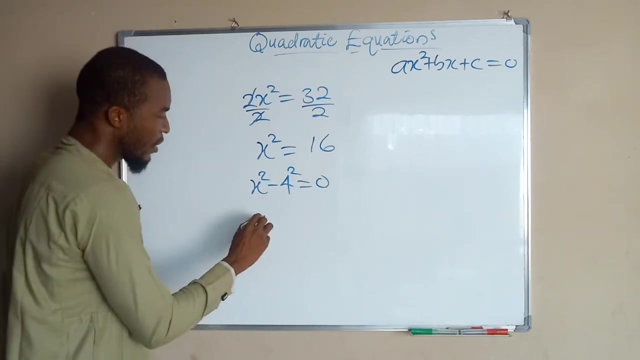 16 and this can be written as 4 squared, because 4 squared is 16. if you bring it towards the left side, we have x squared minus 4 squared equals to 0. also, we have difference of 2 squares which can be written as x minus 4 multiplied by x. 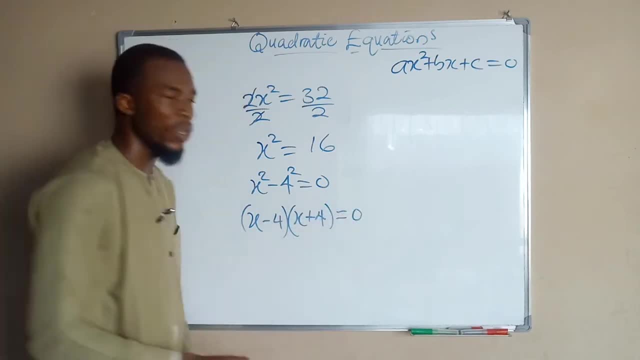 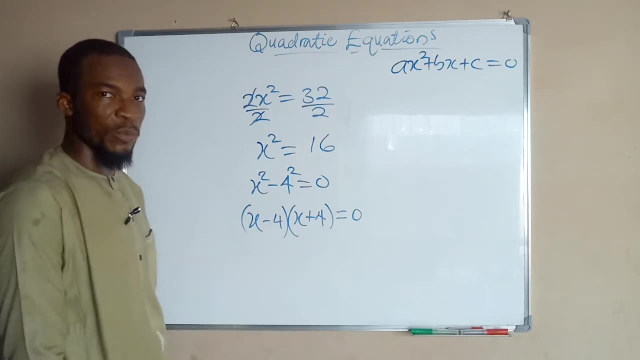 plus 4, and the whole of them equal to 0. to get the roots of this quadratic equation, which is the solution for the quadratic equation, we are going to set each of these factors to be equal to 0. the first factor, x minus 4, equals to 0. this 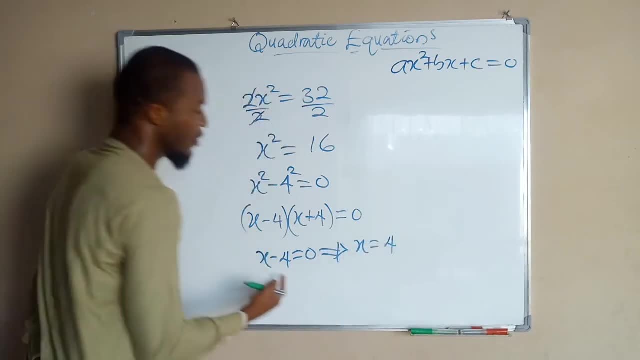 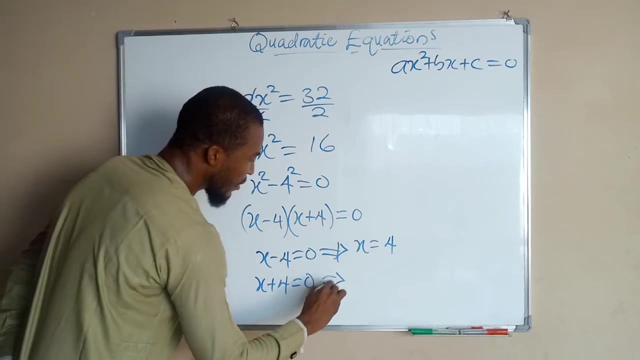 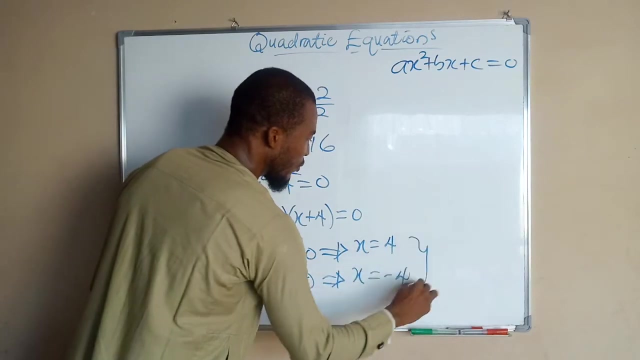 implies that x is equal to 4. for this equation to be true, and for the second factor, x plus 4, equal to 0, this implies that x is equal to negative 4, because negative 4 plus 4 is 0. hence we say the real solution for this quadratic. 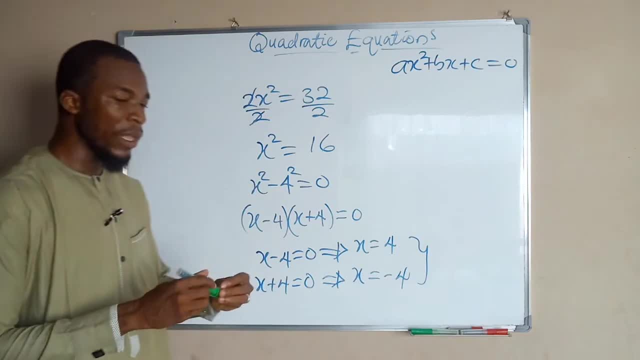 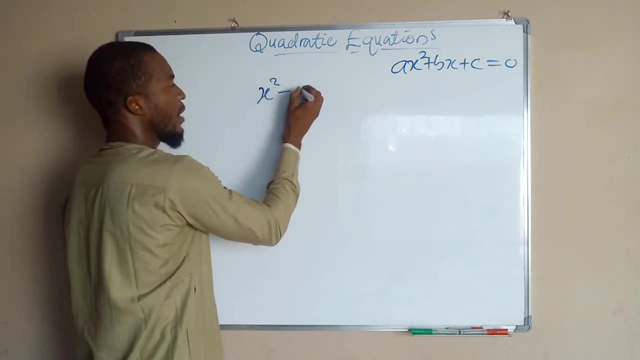 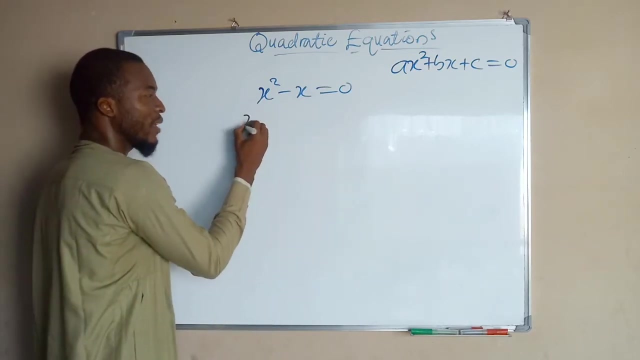 equation are 4 and minus 4. now let us look on to quadratic binomial where we have two times. suppose we have x squared minus x equal to 0. if you can see both times have x in common, which you can factor one of the x out and inside from the first time we have only. 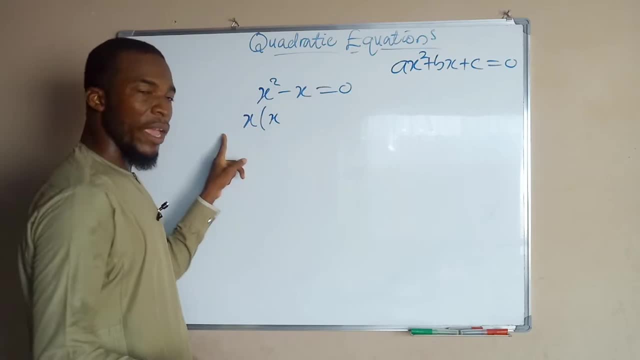 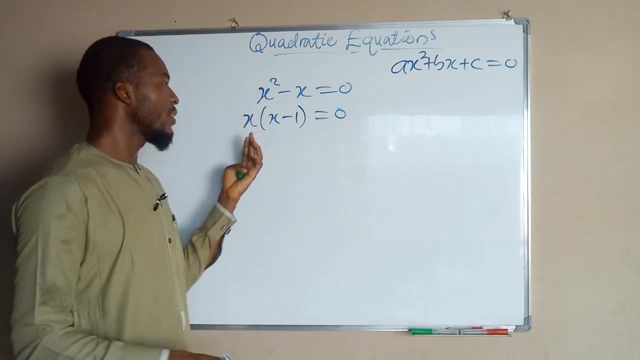 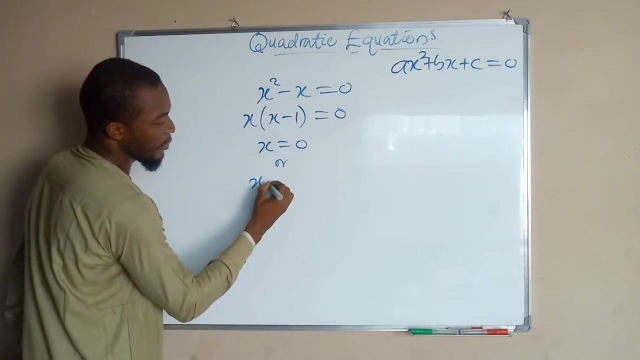 x left and here, since we have factored x out, we are left with 1 and this is equal to 0. hence, we have two factors multiplying each other. we are going to set each one of them to be 0. the first one is x equal to 0 or x minus. 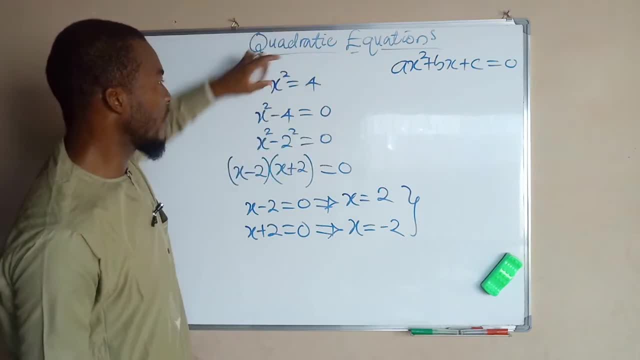 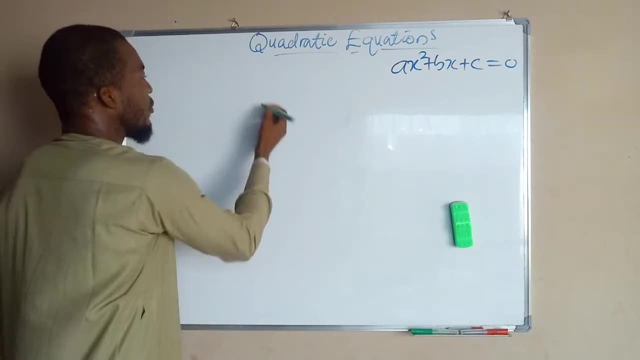 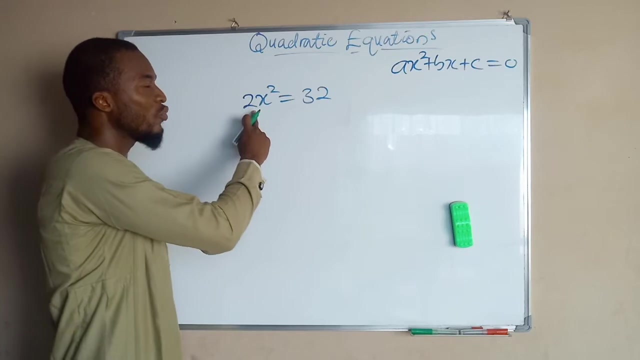 coefficient of x squared is always a. In this equation you can see that a is equal to 1.. This is why we don't have any number attached to x squared. Suppose you have: 2x squared equals to 32.. Here the leading coefficient is equal to 2.. To 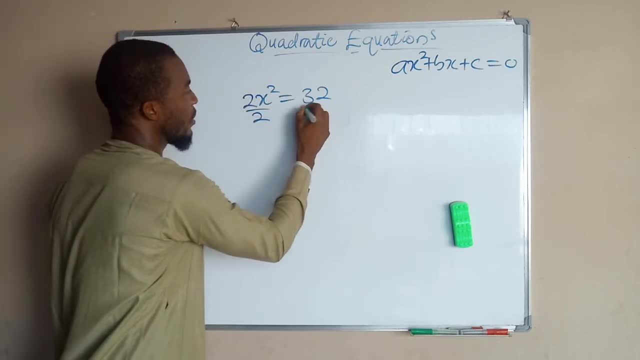 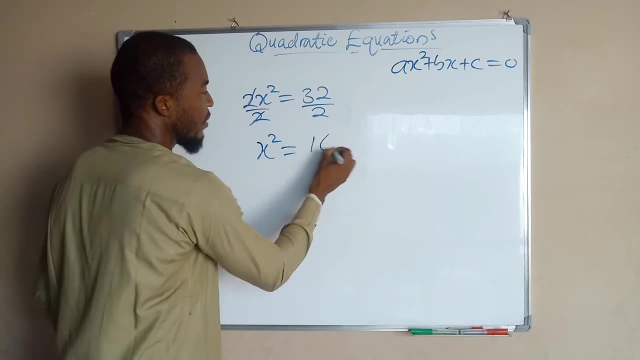 get rid of this 2. you can divide both sides by 2.. So we do divide both sides by 2, which 2 cancel 2, leaving x squared equals to 16, because that is equal to 2.. So we can divide both sides by 2, which 2 cancel 2.. Leaving x squared equals to 16, because that is. 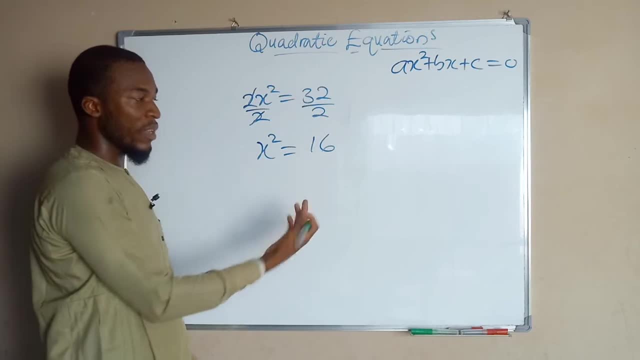 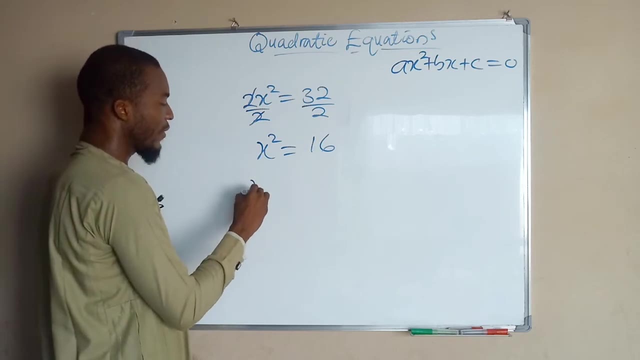 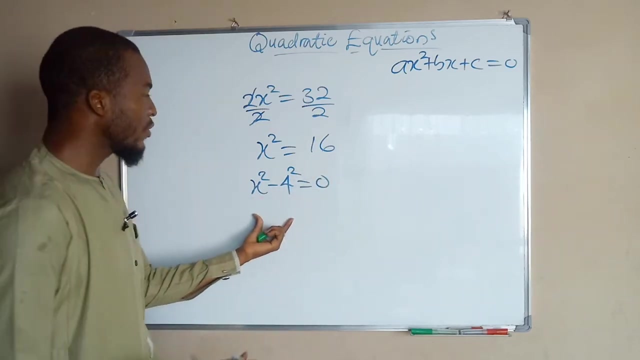 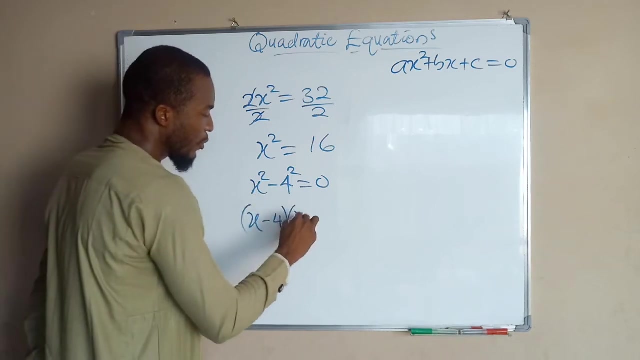 2 divided by 2 is 16. And this can be written as 4 squared, because 4 squared is 16.. If you bring it towards the left side, we have x squared minus 4 squared equals to 0.. Also, we have difference of 2 squares, which can be written as x minus 4 multiplied by x plus. 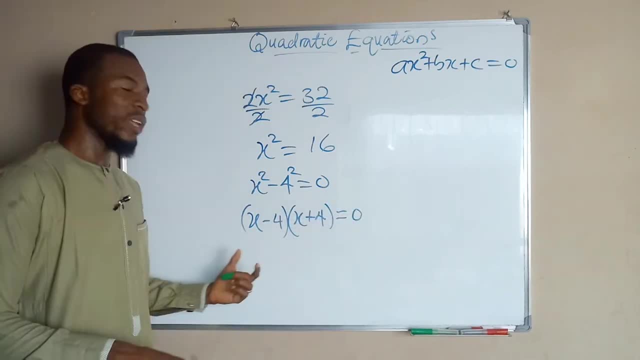 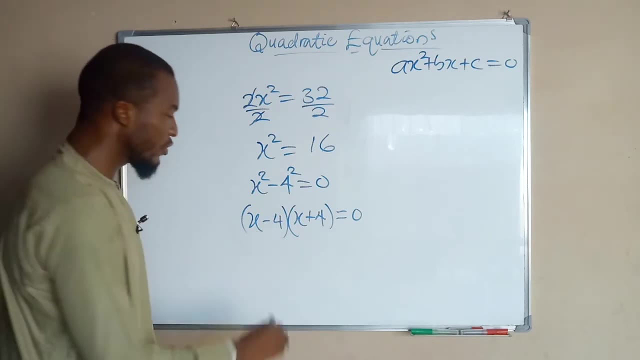 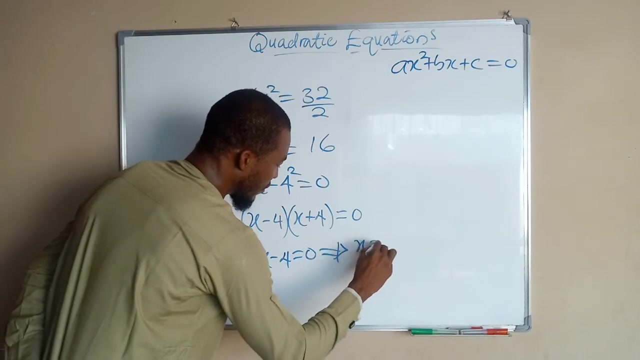 4. And the whole of them equal to 0.. To get the roots of this quadratic equation, which is the solution for the quadratic equation, we are going to set each of these factors to be equal to 0.. The first factor, x minus 4, equals to 0. This implies that x is equal. 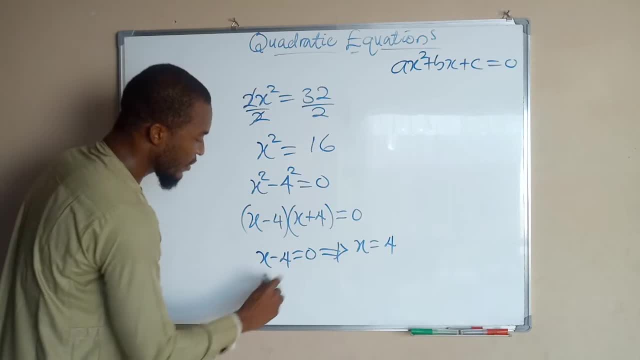 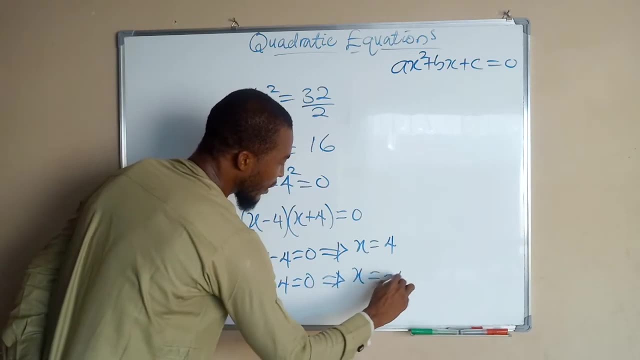 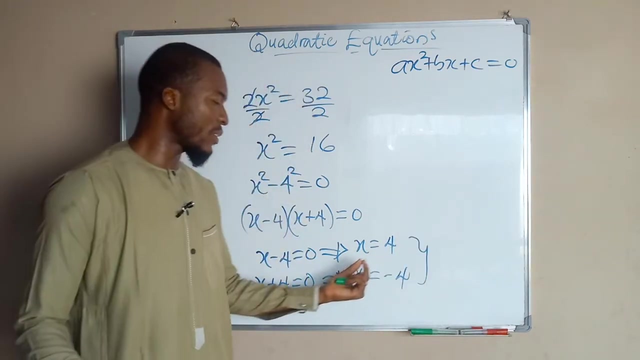 to 4 for this equation to be true, And for the second factor, x plus 4, equals to 0. This implies that x is equal to negative 4.. Because negative 4 is equal to negative 4. And so 4 plus 4 is 0. Hence we say the real solution for this quadratic equation are 4 and negative. 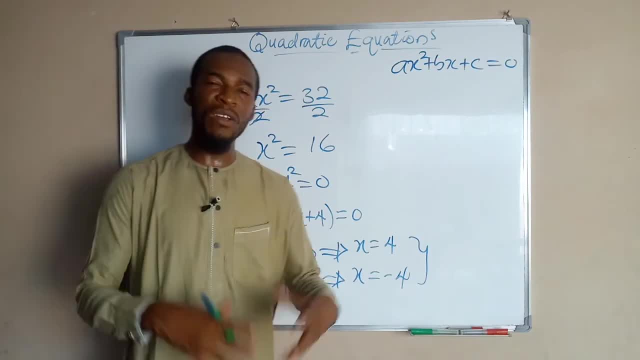 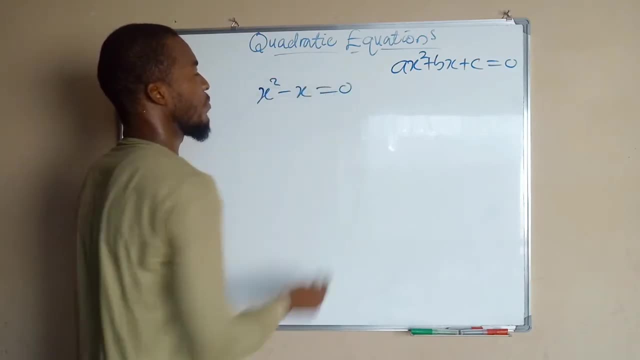 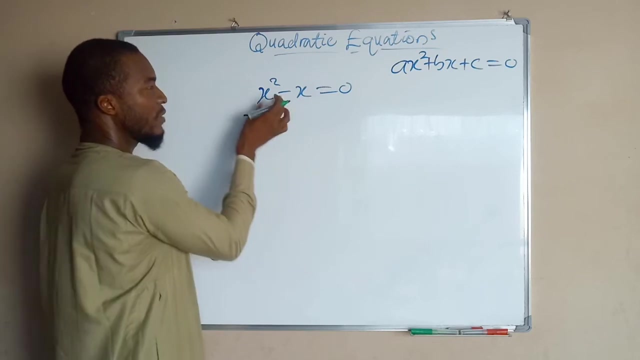 4.. Now let us look on to quadratic binomial where we have two times. Suppose we have x squared minus x equals to 0. If you can see, both times have x in common, which you can factor one of the x out And inside. from the first term we have only x left And here, since 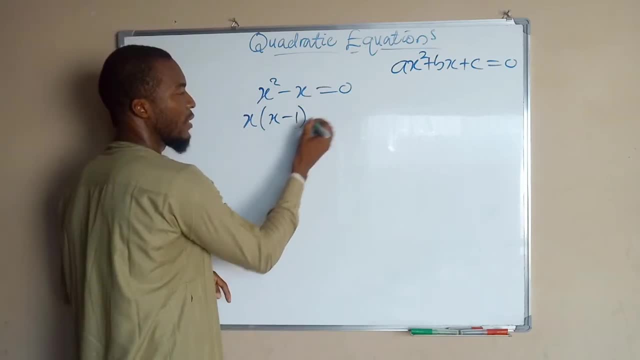 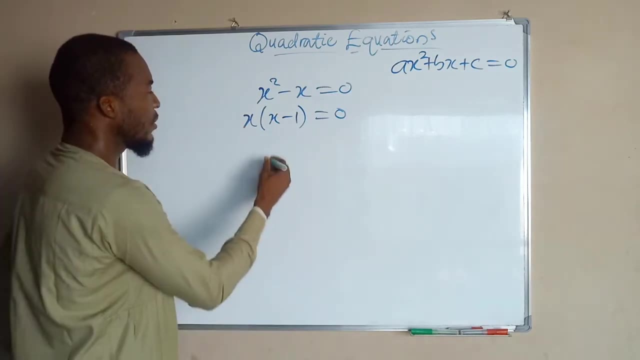 we have factored x out, we have x squared minus x squared, So we have x squared minus x squared minus x squared, So we are left with 1. And this is equal to 0.. Hence we have two factors multiplying each other. We are going to set each one of them to be 0.. 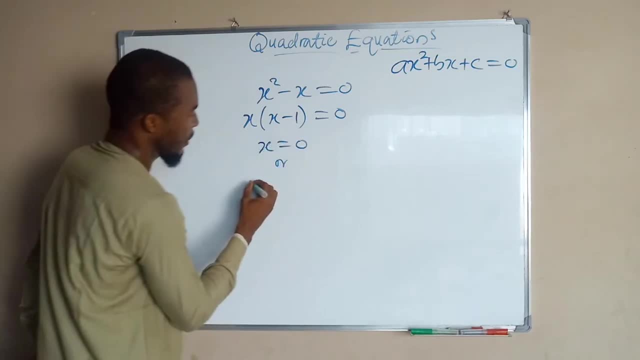 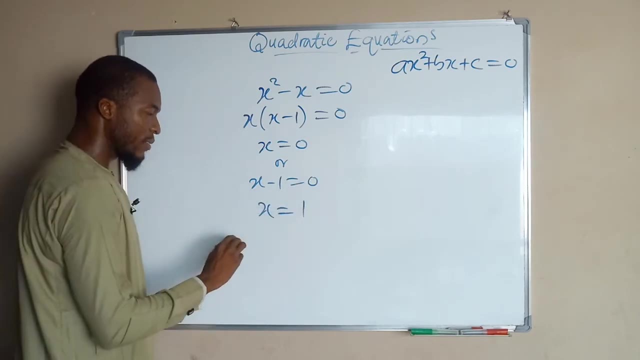 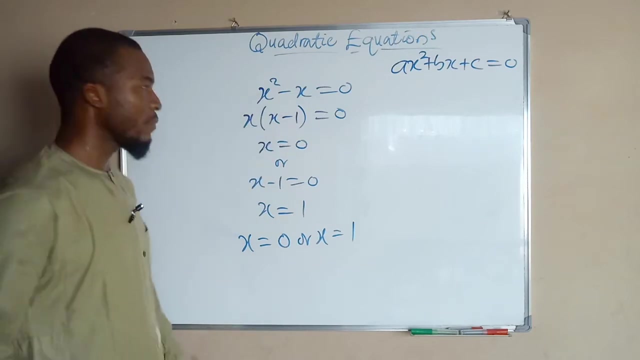 The first one is x equal to 0, or x minus 1 equal to 0,, which implies that x is equal to positive 1.. Hence, x is either equal to 0, or x equal to positive 1 for this equation to be true. Now let us look on to another formula. So this is the final equation, And 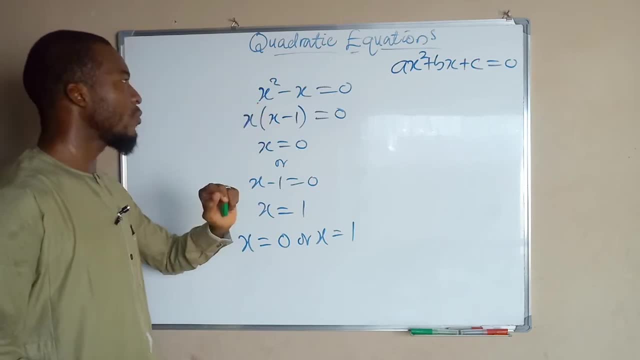 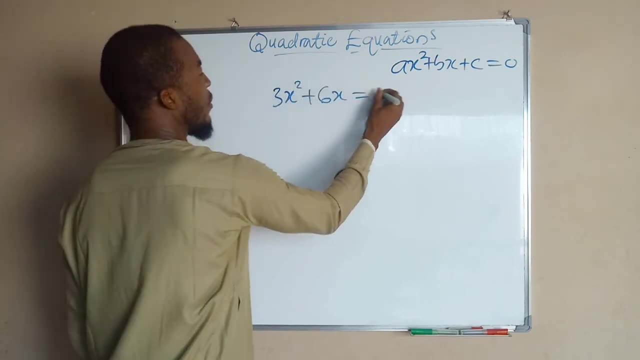 we are left with 1. And this is equal to 0. Hence we have two factors multiplying each, in which the leading coefficient is not equal to 1.. Suppose we have 3x squared plus 6x equal to 0.. To factorize this expression: 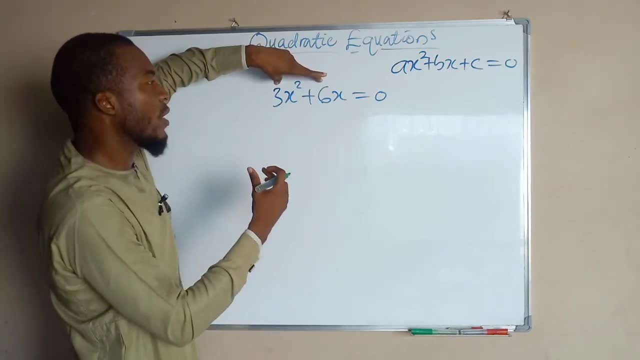 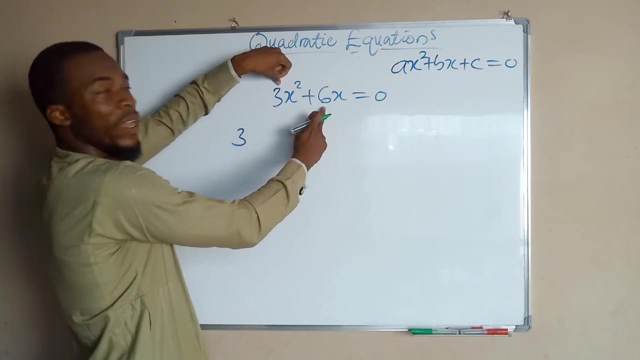 we are going to compare the two numbers and look at their highest common factor, which among them we have 3,, because 3 can go into 3 as well as 6.. Then we look upon the x's, For here they have x in common. 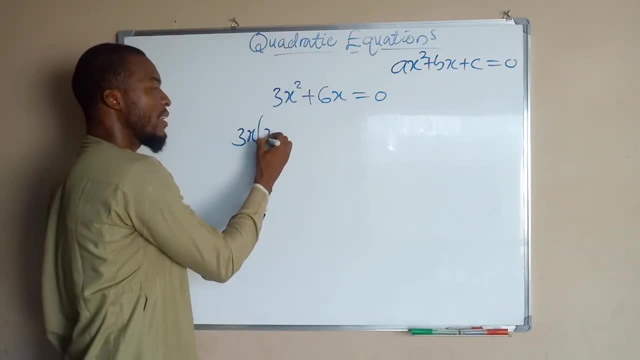 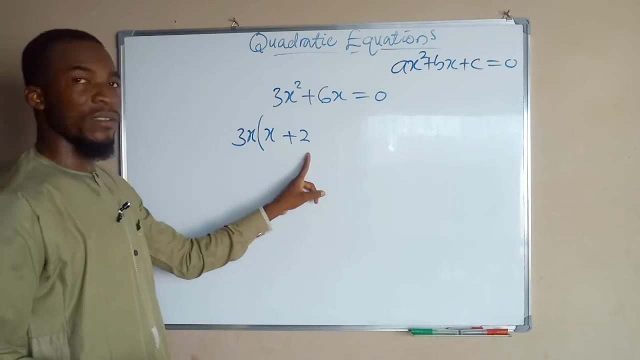 so we have 3x out. From the first term we have only x, And from the second term we have only 2 left, because 6x divided by 3x is equal to 2.. And all of this equal to 0.. 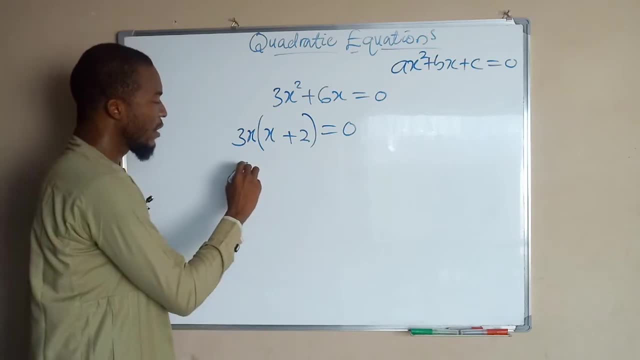 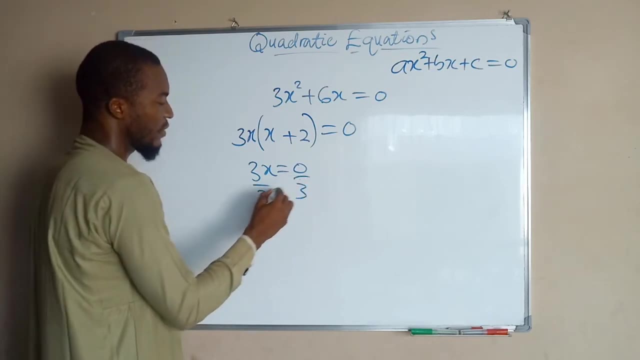 We are going to set each of these factors to be equal to 0.. The first factor is 3x equal to 0.. By dividing both sides by 3, still x cancels. So xx equal to 0 divided by 3, which is still 0. 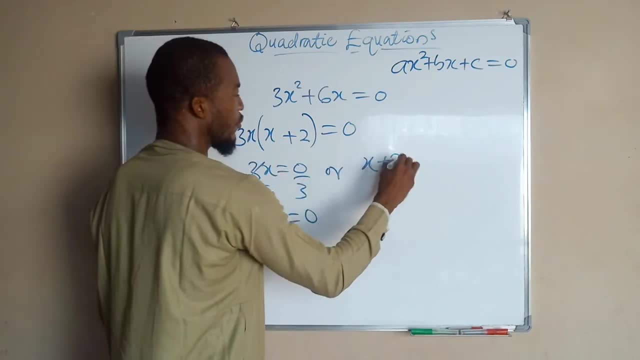 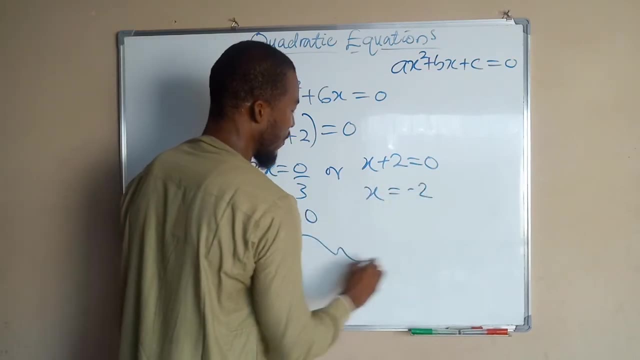 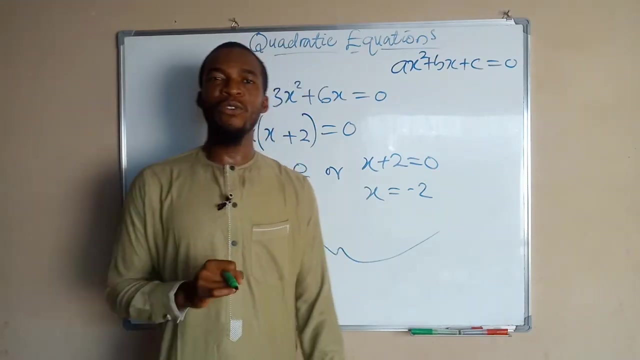 O. The second factor, which is x plus 2, equals to 0. This implies that x is equal to negative 2.. Hence, these are our solutions: x equal to 0 or x equal to negative 2.. So now let us look on to how to factorize quadratic trinomials. 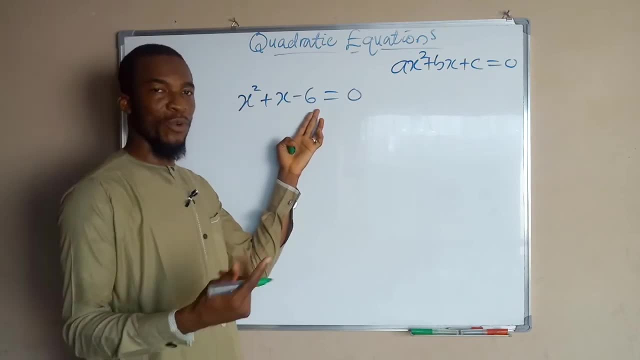 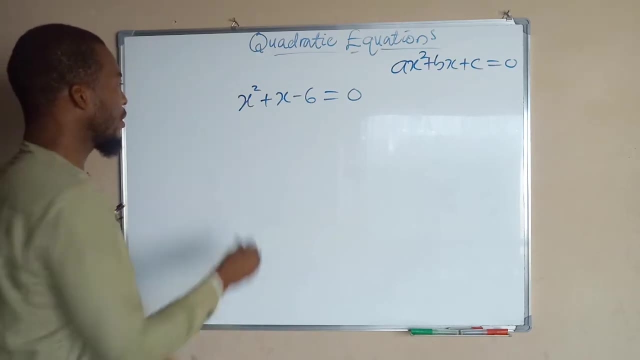 This time around we have 3 times instead of 2 or 1.. The simplest way to factorize an expression in this form, where the leading coefficient is 1, is to have 2 brackets first, and each one of them is equal to 0.. 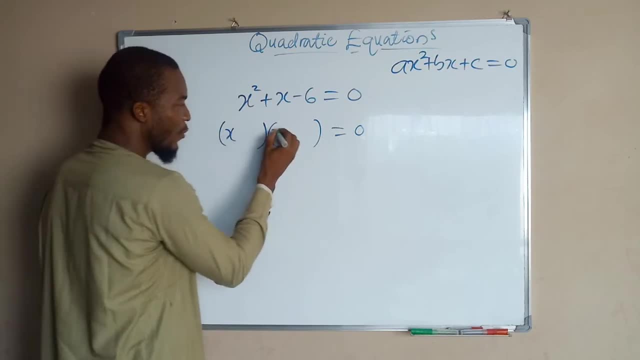 We have x here. we have x here. What we are going to think of. we are going to think of 2 factors, of negative 6, which, when you add them together, you get positive 1, which is the coefficient of the middle term, which is x. 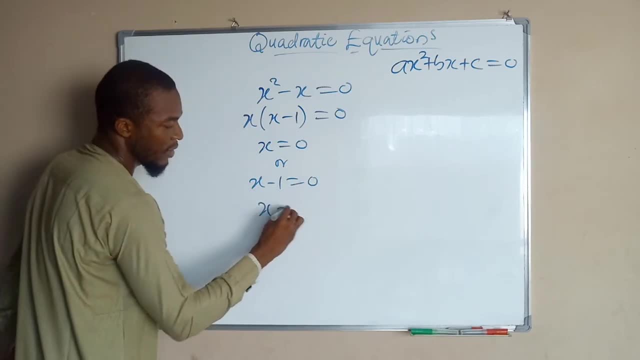 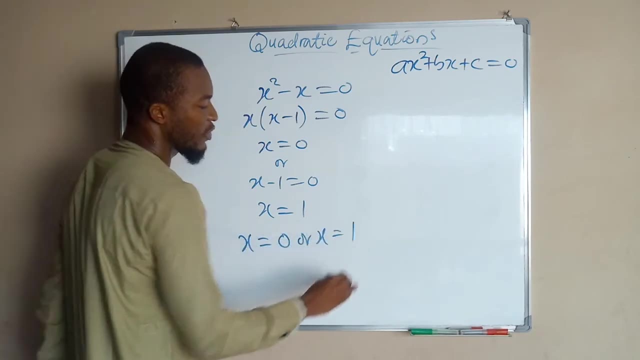 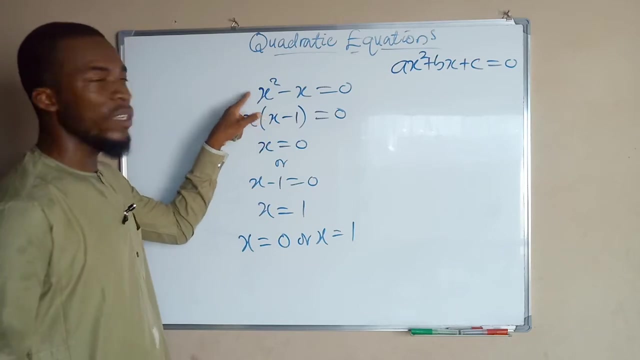 1 equal to 0, which implies that x is equal to positive 1. hence, x is either equal to 0 or x equal to positive one. for this equation to be true, now let us look on to another form in which the leading coefficient is not equal to 1.. 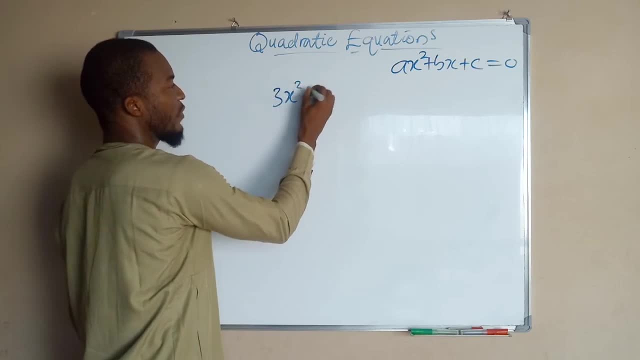 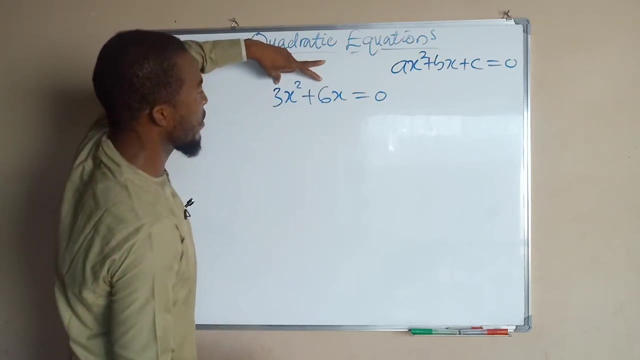 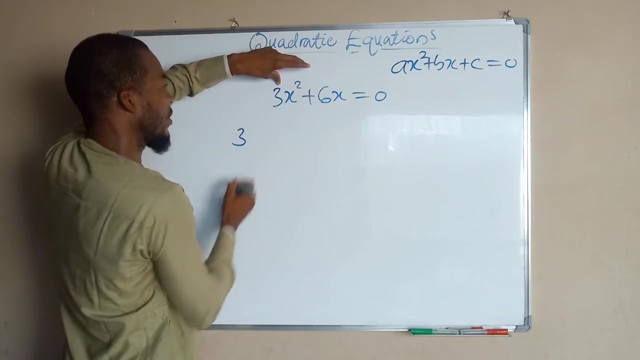 we have 3x squared plus 6x, equal to 0.. To factorize this expression, we are going to compare the two numbers and look at their highest common factor, which among them we have 3, because 3 can go into 3 as well as 6.. Then we look upon the x's, for here they. 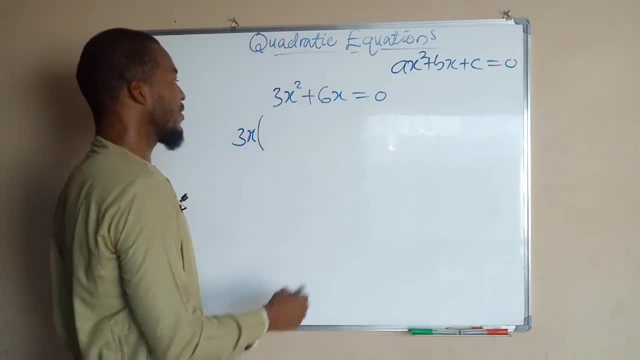 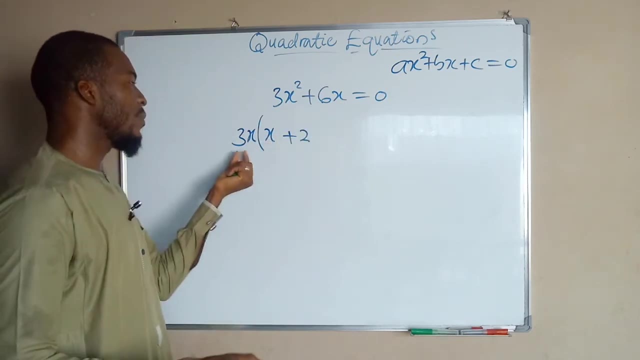 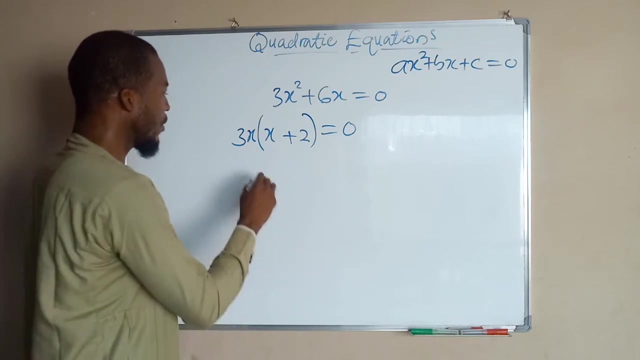 have x in common, so we have 3x out. From the first term we have only x and from the second term we have only 2 left, because 6x divided by 3x is equal to 2 and the whole of this equal to 0. We are going to set each of these factors to be equal to 0.. The first factor: 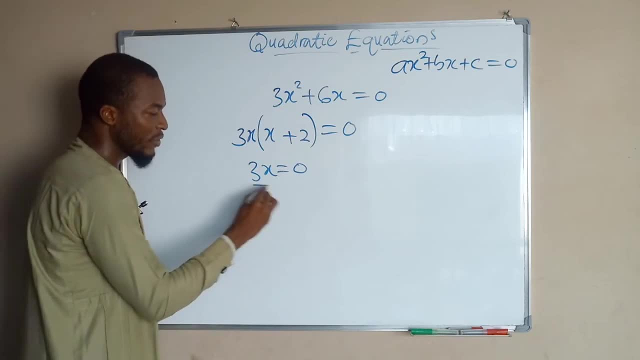 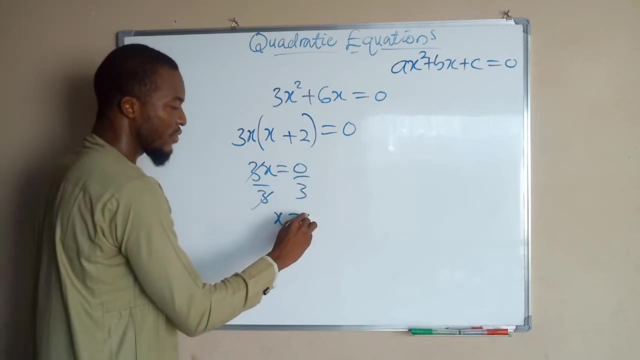 is 3x equal to 0.. By dividing both sides by 3, still x cancel x. x equal to 0. divided by 3, which is still 0.. Or the second factor, which is x plus 2, equals to 0.. 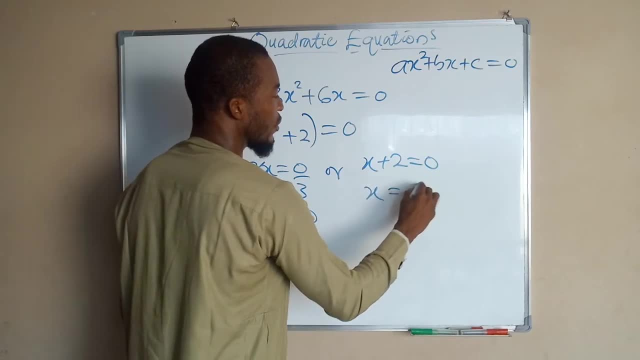 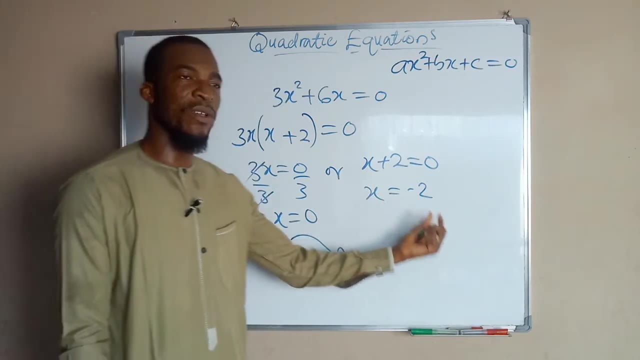 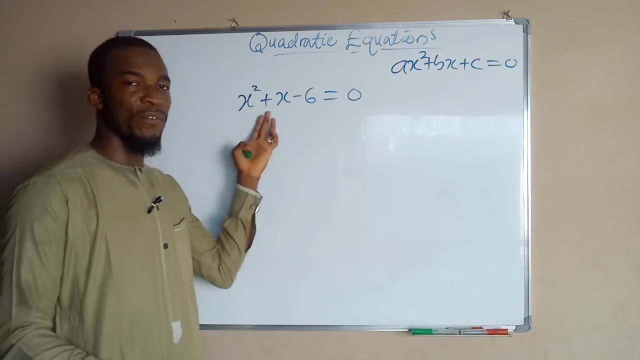 This implies that x is equal to negative 2.. Hence, these are our solutions: x equal to 0 or x equal to negative 2.. So now let us look onto how to factorize quadratic trinomials. This time around we have 3 times instead of 2 or 1.. The simplest way to factorize an expression: 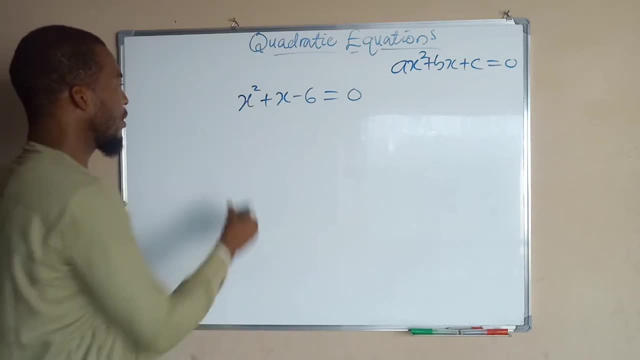 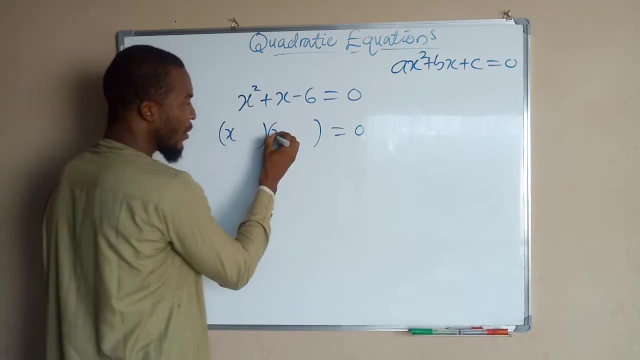 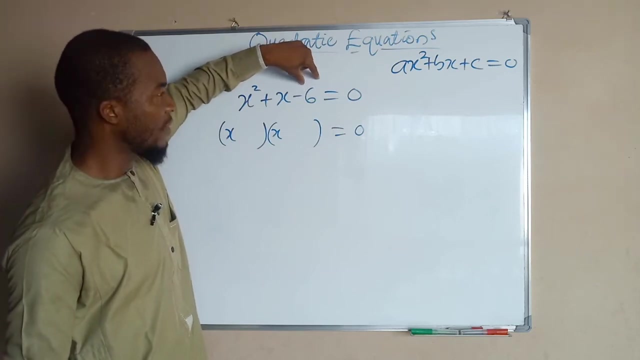 in this form, where the leading coefficient is 1, is to have 2 brackets. first We have x here and x here. What we are going to think of? we are going to think of two factors of negative 6 which, when you add them together, you get positive 1, which is the co-. 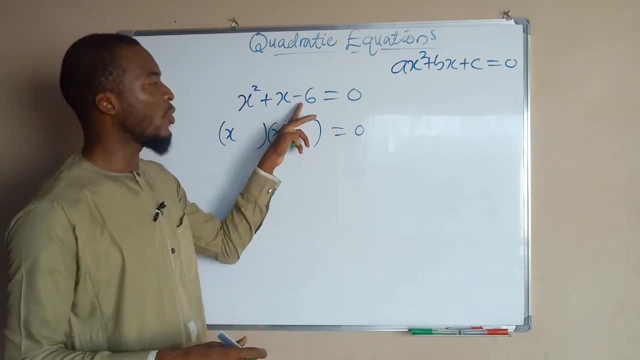 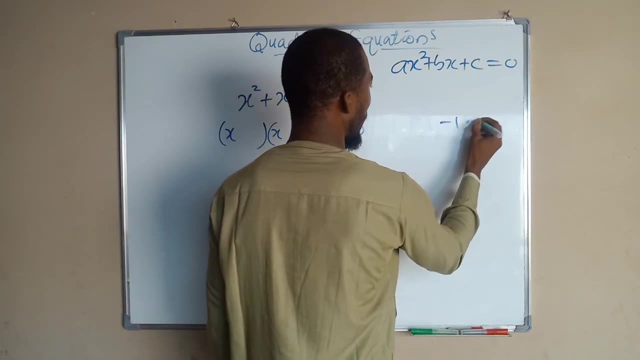 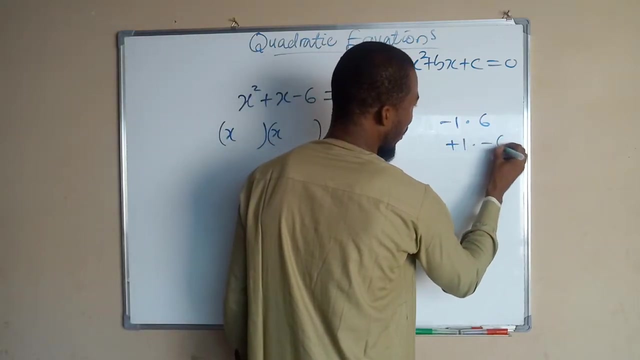 vision of the middle term, which is x. So let us first of all list out the factors of negative 6.. We have negative 1 multiplied by 6 will give us negative 6.. We have negative 1 multiplied by negative 6 and we have positive 1 multiplied by negative 6 will still give us negative. 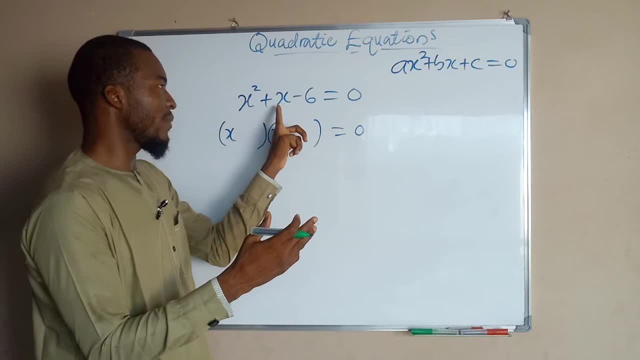 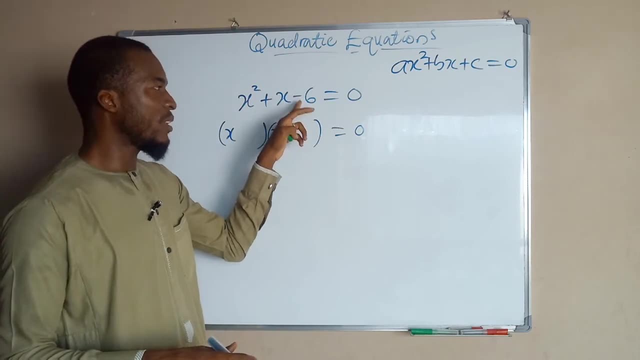 So let us first of all list out the factors of negative 6.. We have negative 1, multiplied by 2,, which is negative 1, which is negative 1, multiplied by 2,, which is negative 1, multiplied by 2,, which is negative 1,. 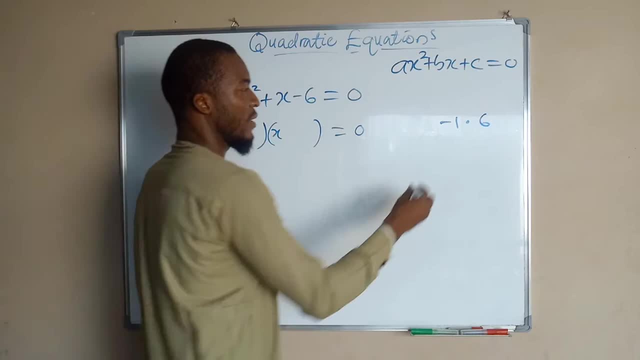 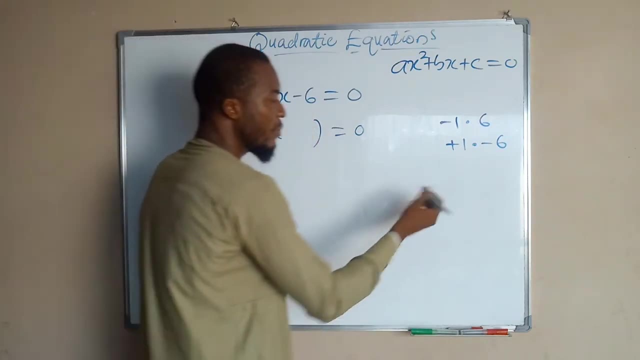 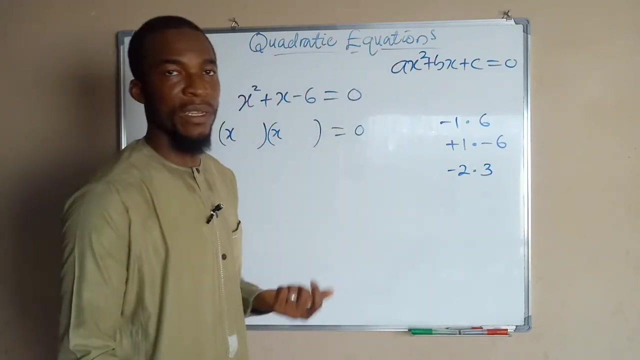 multiplied by 6, will give us negative 6.. And we have positive 1, multiplied by negative 6, will still give us negative 6.. We may have negative 2 multiplied by positive 3,, still it will give us negative 6.. 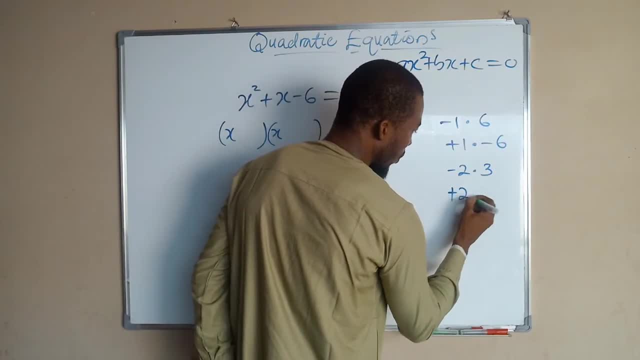 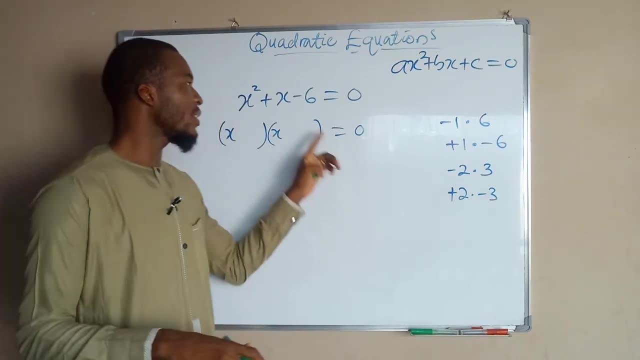 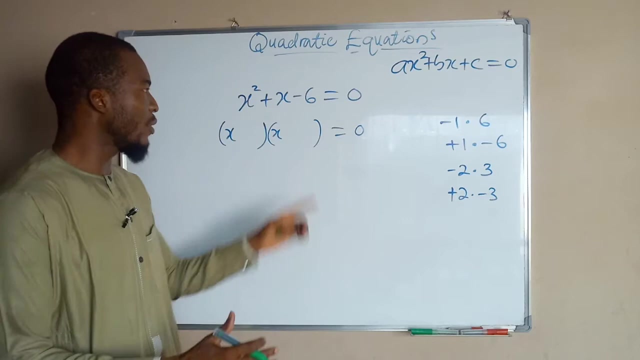 We may have a positive 2 multiplying a negative 3. All these set of numbers, if you multiply them together, you get negative 6. So you are going to decide which group among these 4 groups that, if you add them together, 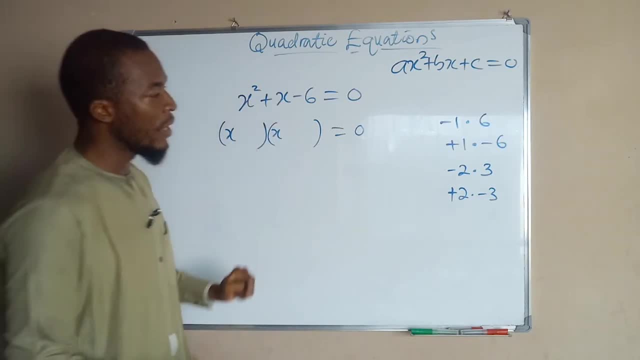 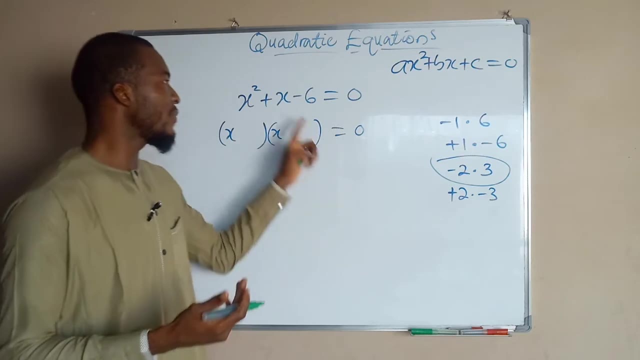 you are going to get a positive 1,, which is the coefficient of the middle term. If you can see this group- negative 2, if you add it to positive 3, it will give us positive 1.. So these are the numbers we are going to use. 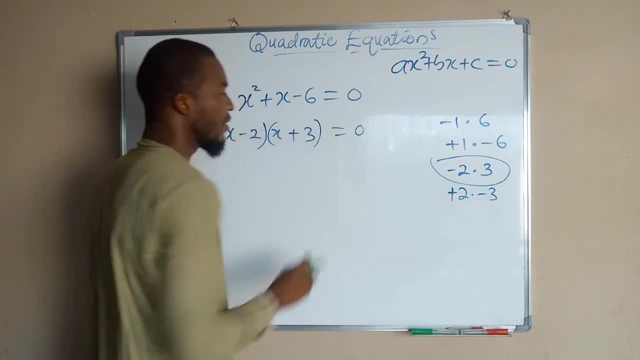 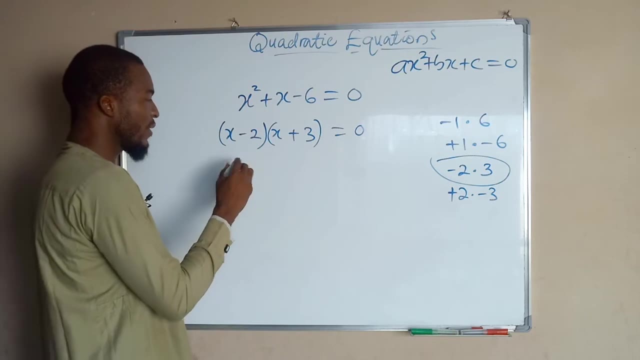 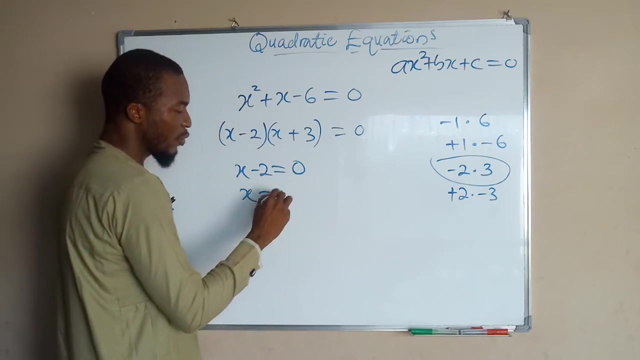 We have negative 2 and positive 3.. Hence we have 2 factors in this quadratic equation. We are going to set each one of them to be equal to 0.. The first one is: x-2 equals to 0. This implies that 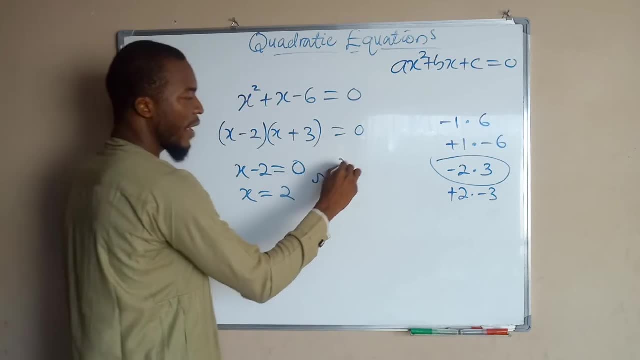 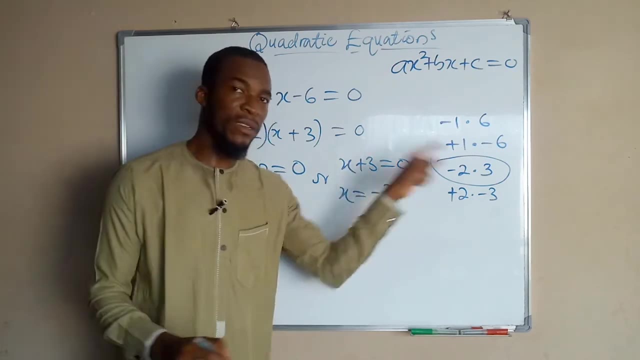 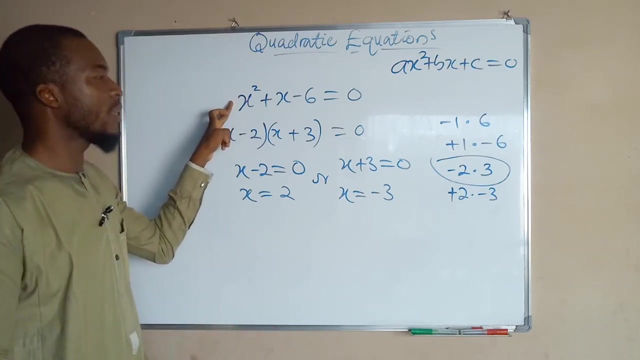 x is equal to positive 2.. Or x plus 3 equals to 0. This implies that x is equal to negative 3 if you take 3 to the other side. This is how to solve a quadratic trinomial. Now let us look onto another form. 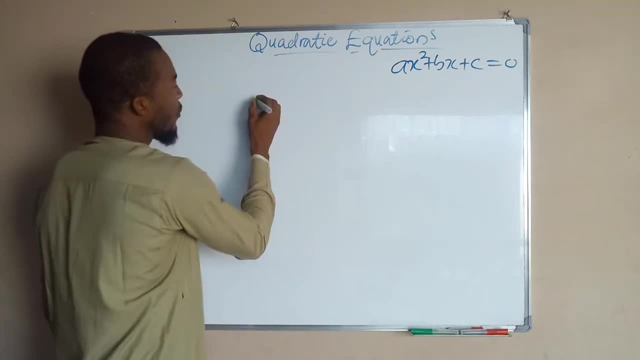 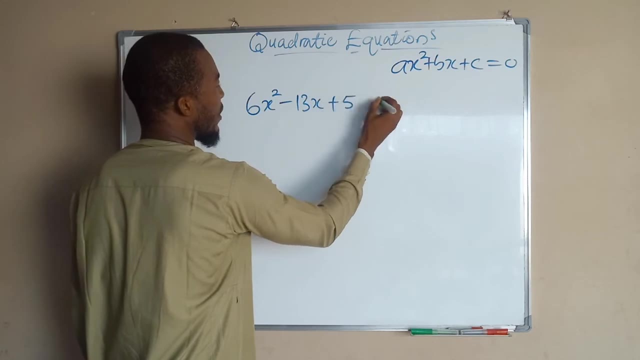 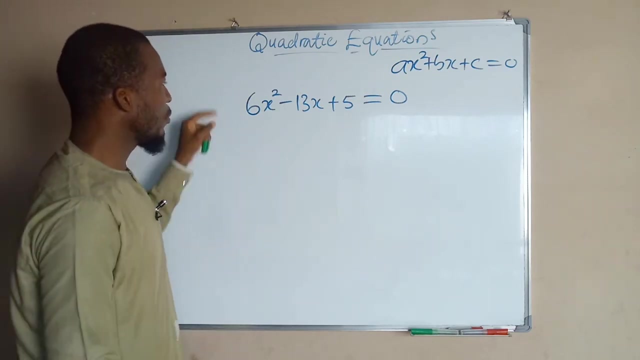 in which the leading coefficient is not 1.. Suppose we have 6x squared minus 13x plus 5 equals 0. First thing you need to do here: you are going to multiply the leading coefficient with the constant term, which is now going to be 6, multiplied by 5. 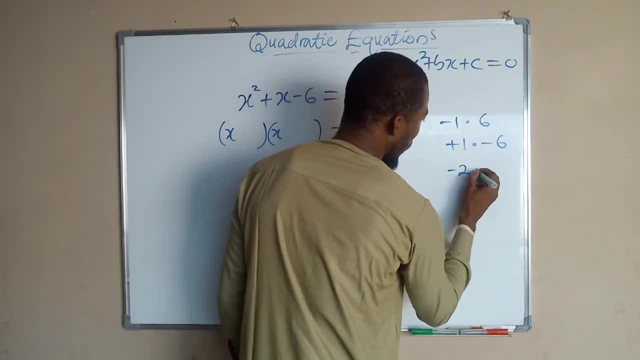 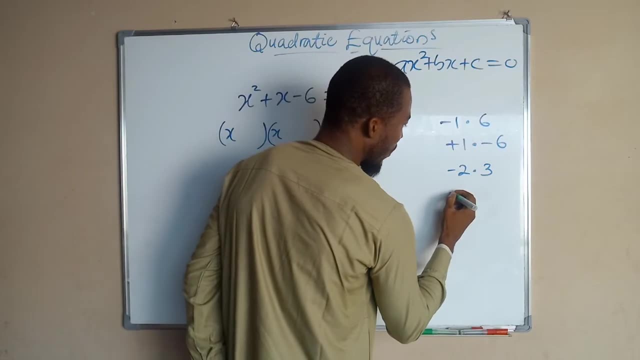 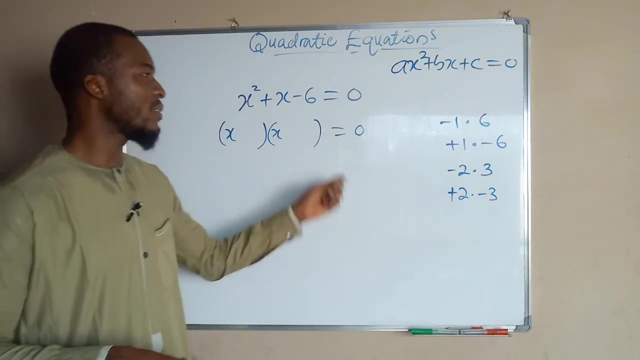 6. We may have negative 2 multiplied by positive 3. Still, it will give us negative 6. We may have a positive 2 multiplying a negative 3. All these set of numbers, if you multiply them together, you get negative 6.. So you are going to decide which group among these four. 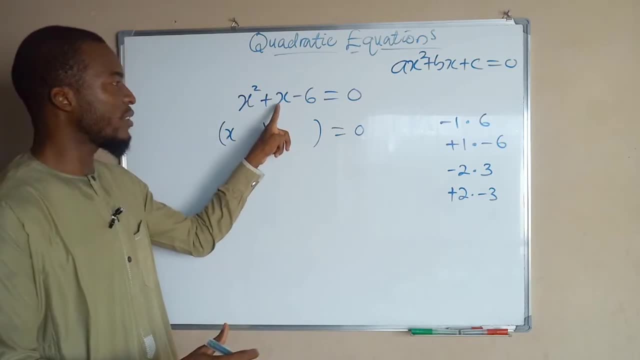 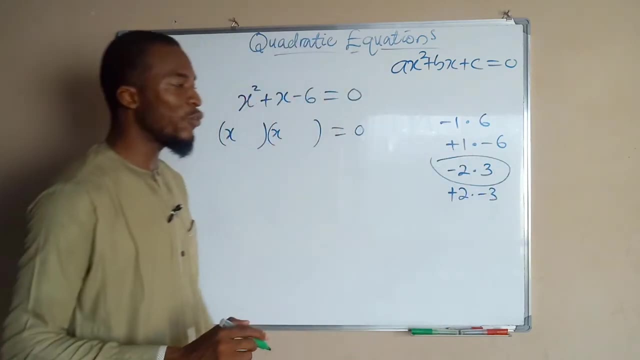 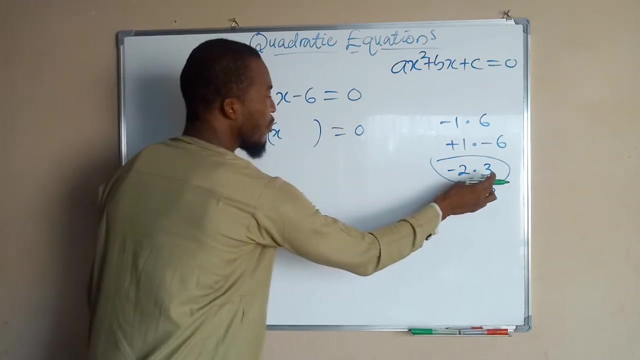 groups that if you add them together, you are going to get a positive 1, which is the coefficient of the middle term. If you can see this group- negative 2. if you add it to positive 3, it will give us positive 1.. So these are the numbers we are going to use. We have negative. 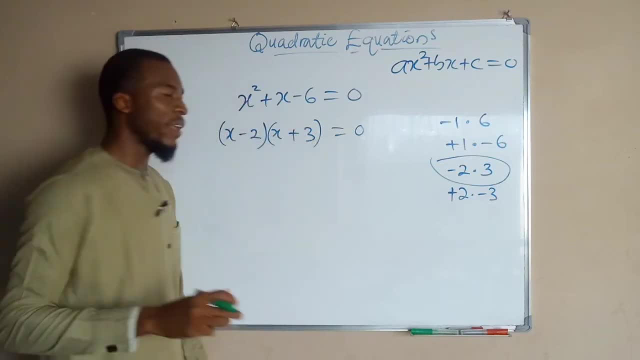 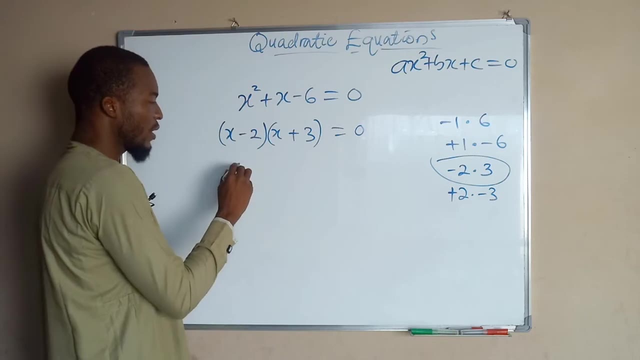 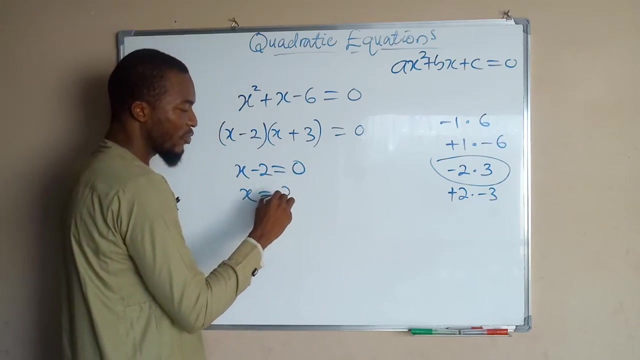 2 and positive 3.. Hence we have two factors of this quadratic equation. We are going to set each one of them to be equal to 0.. x minus 2 equals to 0. This implies that x is equal to positive 2.. Or x plus 3 equals. 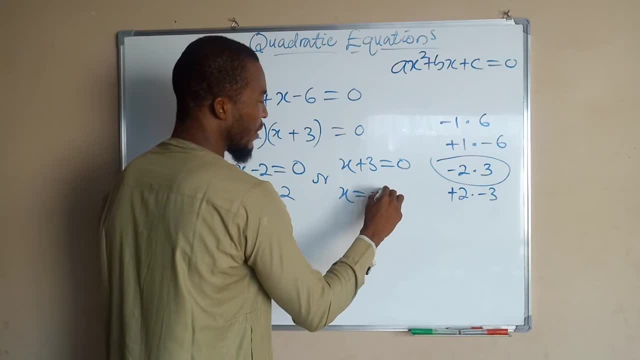 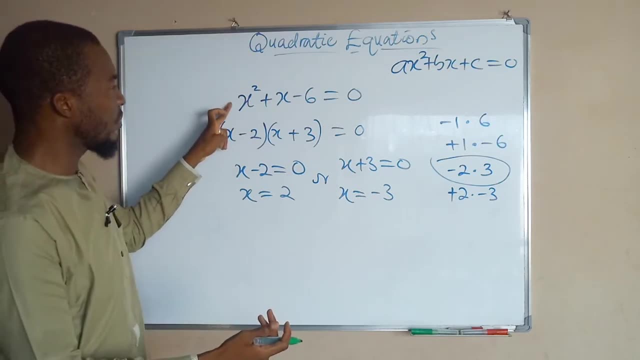 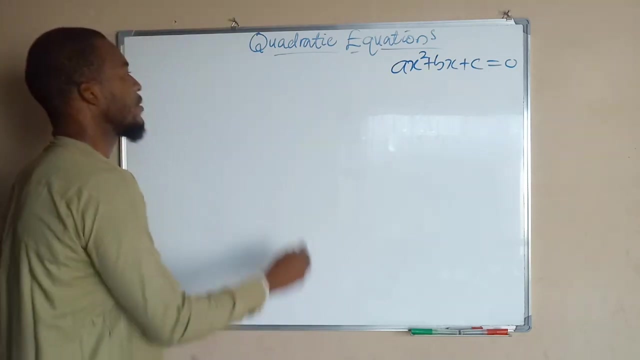 to 0. This implies that x is equal to negative 3 if you take 3 to the other side. This is how to solve a quadratic trinomial in which the leading coefficient is 1.. Now let us look on to another form in which the leading coefficient is not 1.. 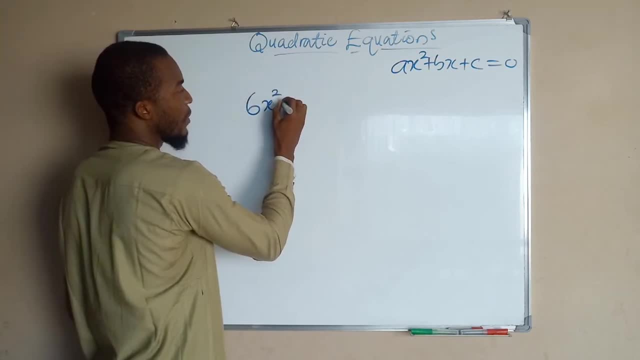 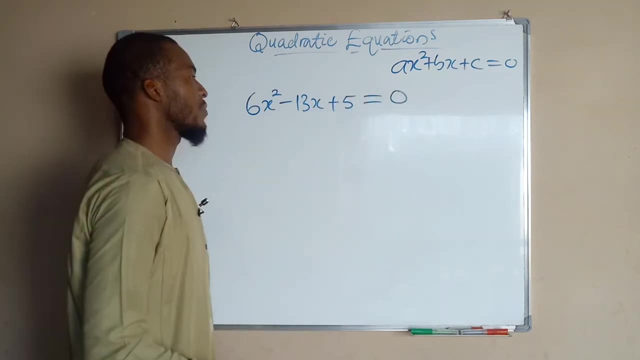 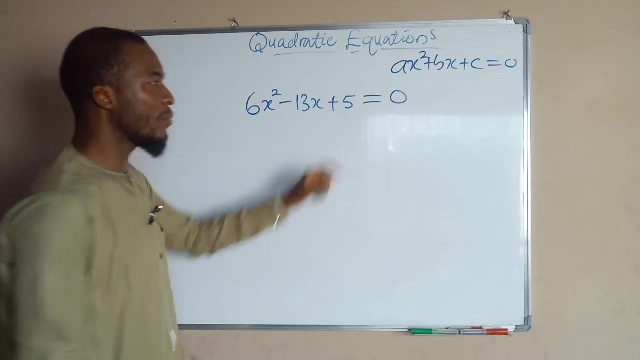 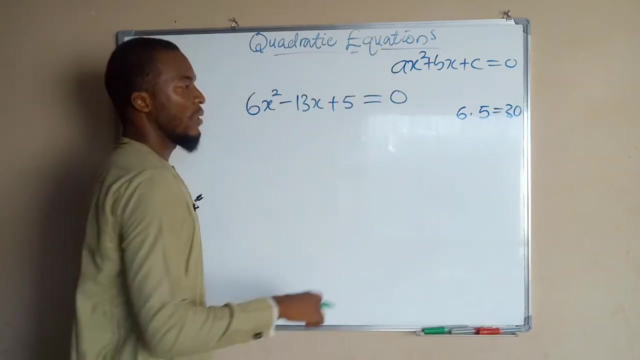 Suppose we have 6x squared minus 13x plus 5 equals 0.. First thing you need to do here: you are going to multiply the leading coefficient with the constant tau, which is now going to be 6, multiplied by 5, and this is equal to 30.. Now we are going to find the two factors. 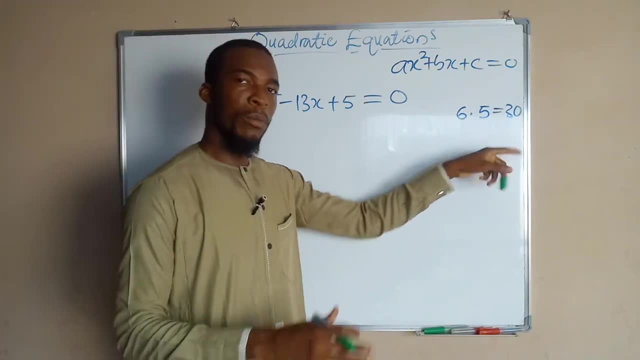 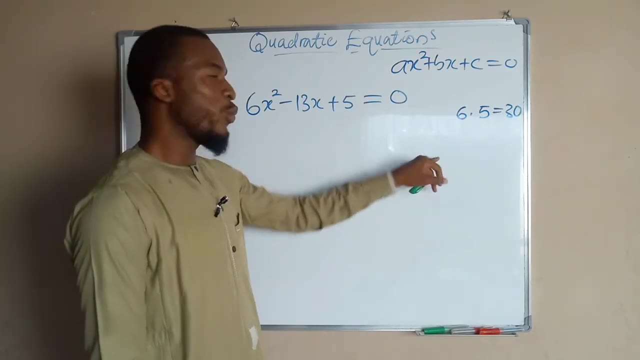 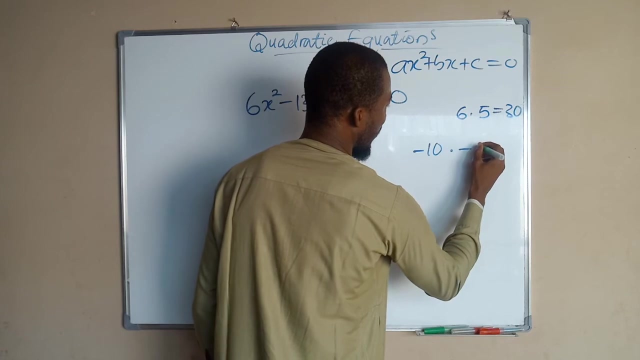 of 30, which, when we multiply them together, we get 30.. For one added together, we get negative 13, which is the coefficient of the middle term. I don't want to waste much of your time. The factors are going to be negative, 10 and negative. 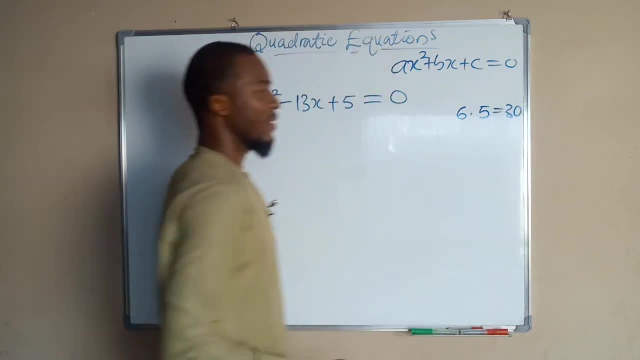 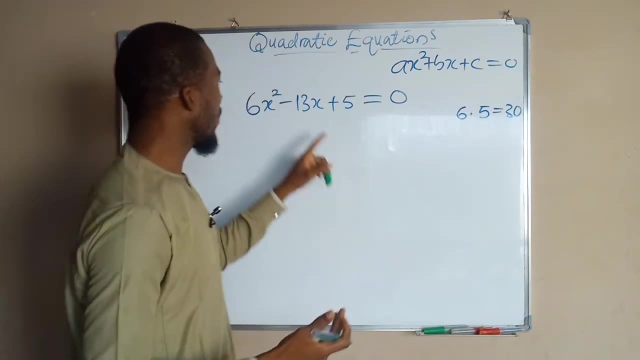 and this is equal to 30. Now we are going to find the 2 factors of 30 which, when we multiply them together, we get 30. But when added together we get negative 13, which is the coefficient of the middle term. I don't want. 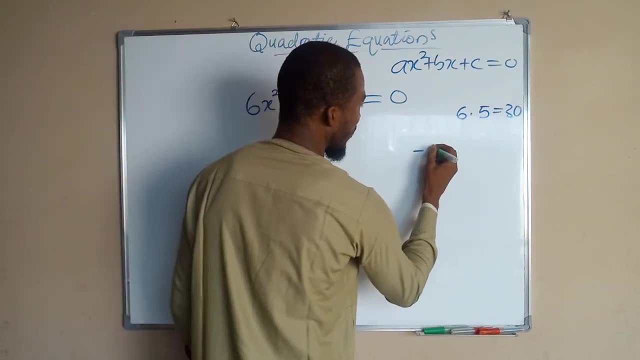 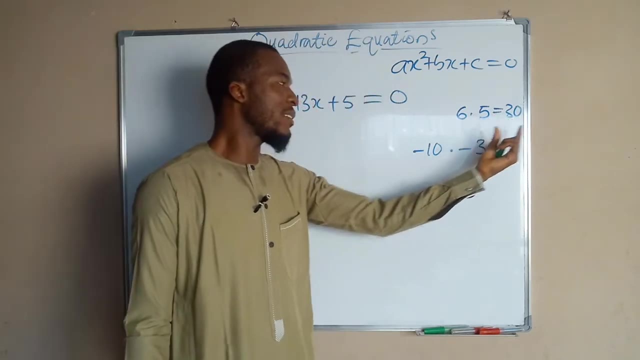 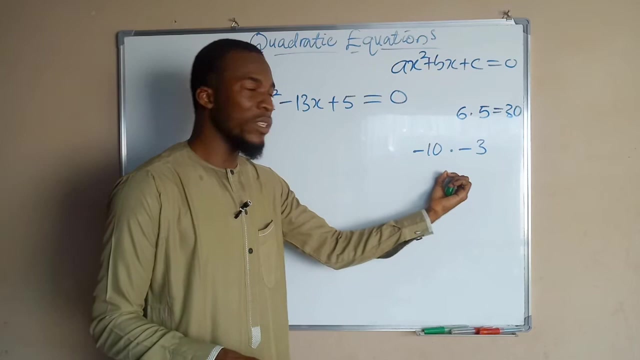 to waste much of your time. The factors are going to be negative 10 and negative 3 because among the 2 factors of 30, this is the only group you can multiply together to get positive 30 and add together, you get negative 13.. 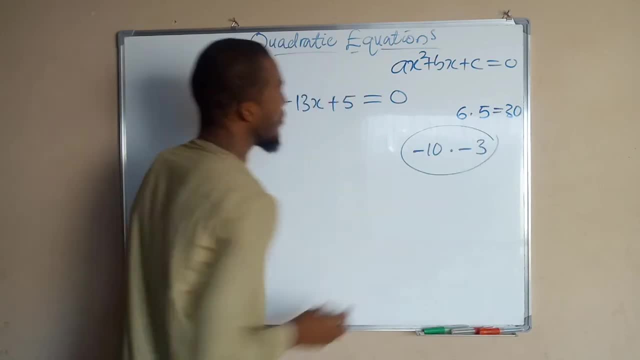 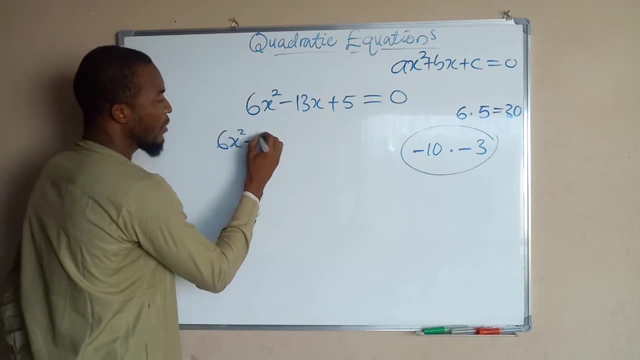 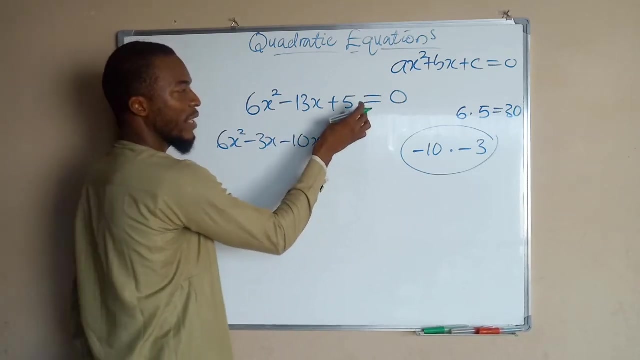 So we are going to replace the middle term with these 2 terms. So we have 6x squared minus 3x. which is this then, minus 10x plus 5, plus the last term, this is equal to 0.. Then we are going to factorize in batches. 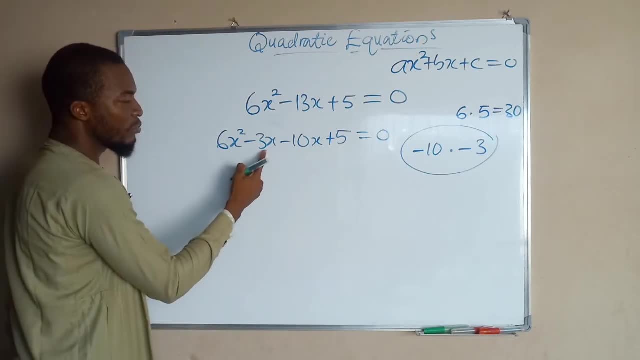 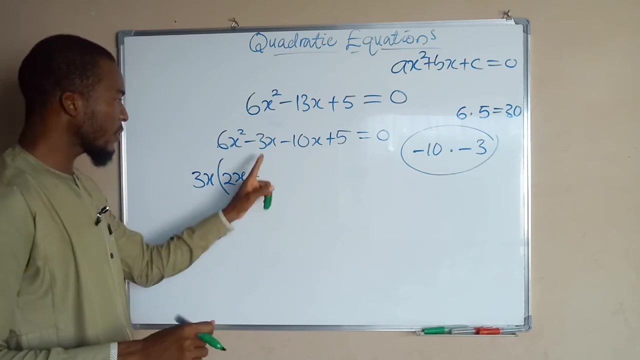 the first 2 and the second 2.. The first 2,. among the numbers, they have 3 in common. so we have 3.. Among the unknown variables, we have x in common From the first term. if you divide this by this, you are going to obtain 2x. 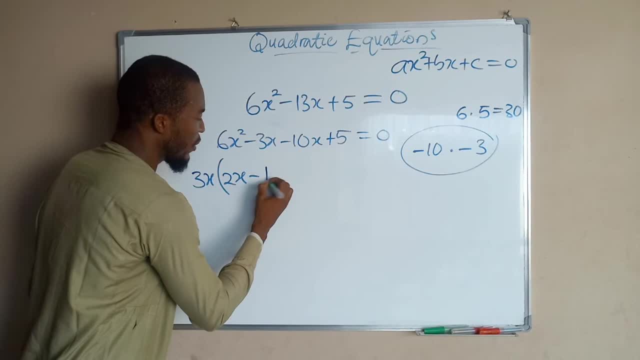 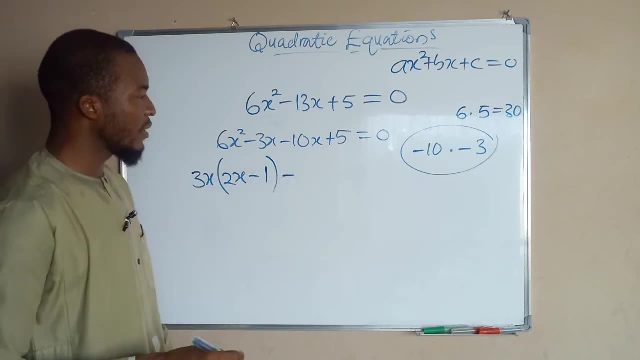 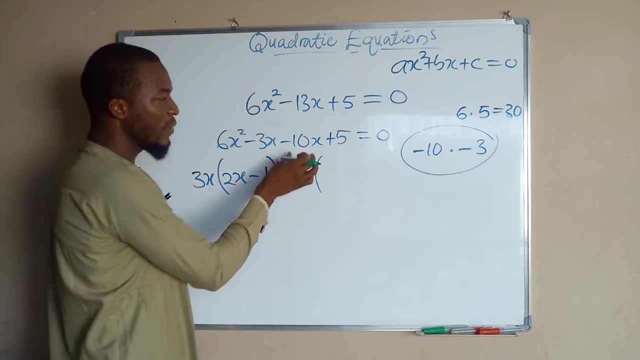 minus. already we have factored 3x out, so we are left with only 1 here. Then you drop your sign, which is minus. among these 2 terms we have 5 in common, so we have 5. In the bracket if you divide negative 10x. 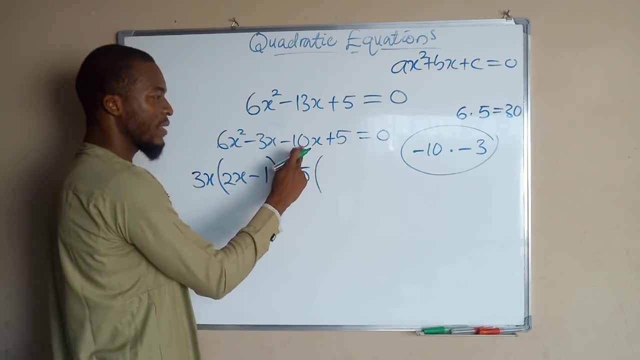 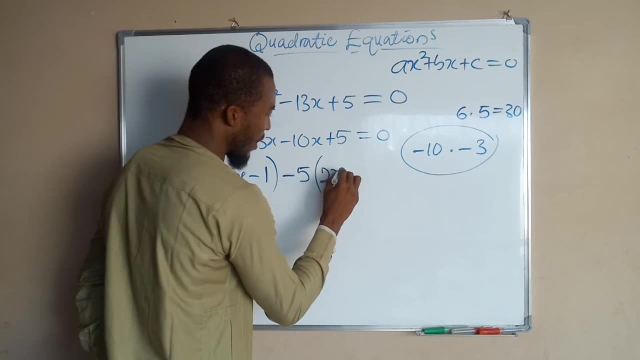 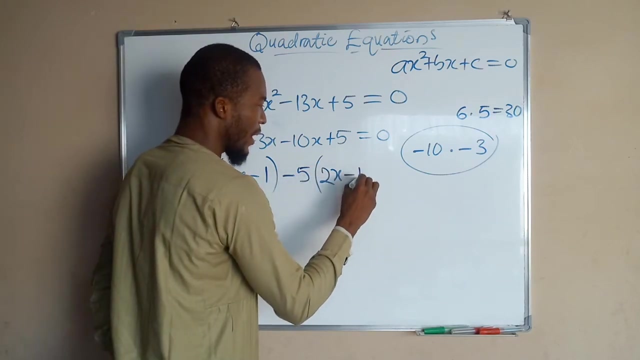 negative will cancel negative. having a positive sign. then 10 divided by 5, we have 2. then x has no x to divide, so we have x. Then 5 divided by negative, 5 is going to make it negative 1. The whole of this equal to 0. 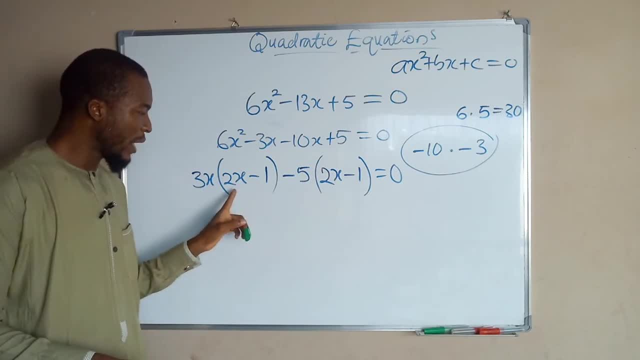 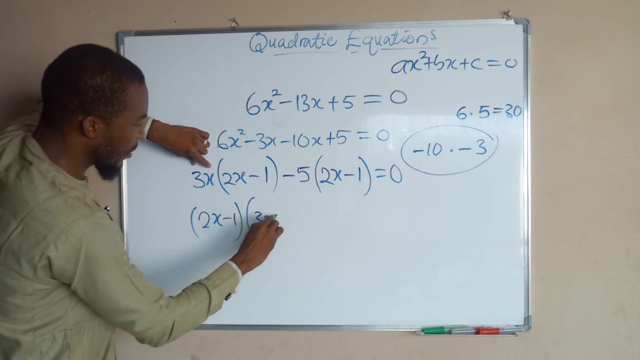 Now, if you look at these 2 terms, all have 2x minus 1 in common, which you can factor out: 2x minus 1. from the first term, we have only 3x left. from the second term, we have only minus 5 left. 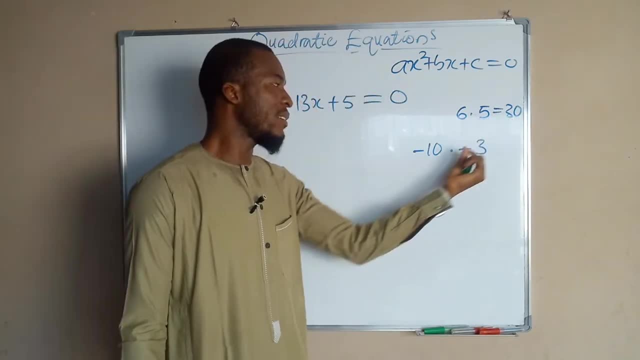 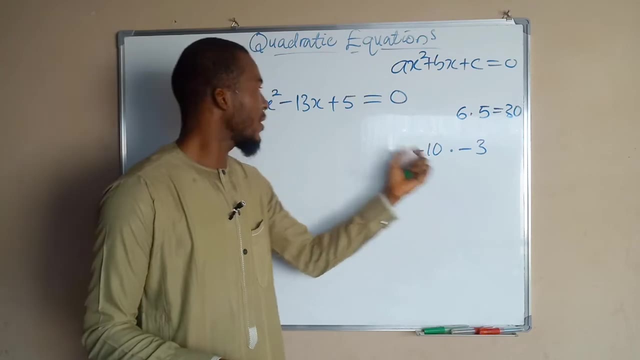 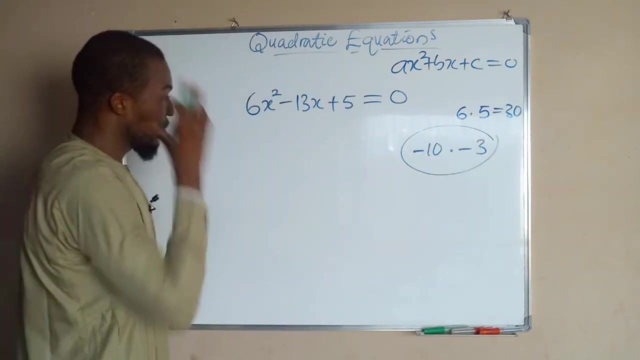 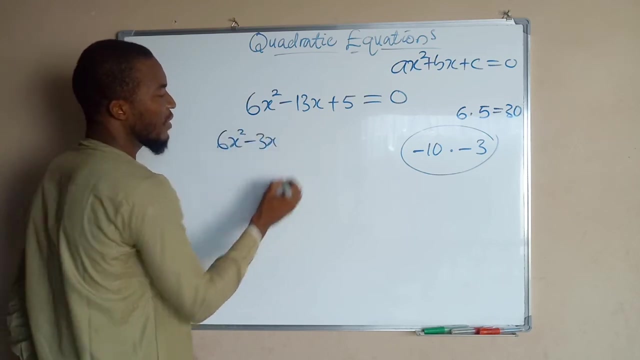 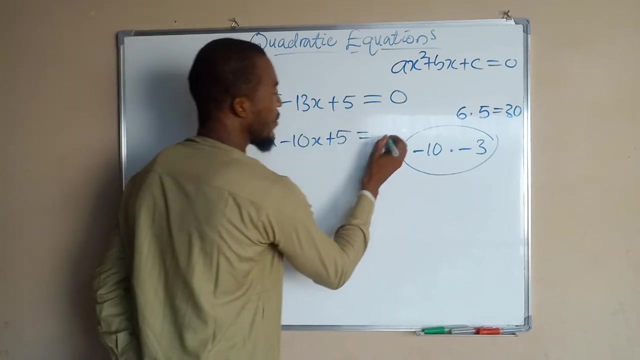 3. Because among the two factors of 30, this is the only group you can multiply together to get positive 30 and add together to get negative 13. So we are going to replace the middle term with these two together. So we have 6x squared minus 3x, which is this then: minus 10x plus 5, plus the last term. 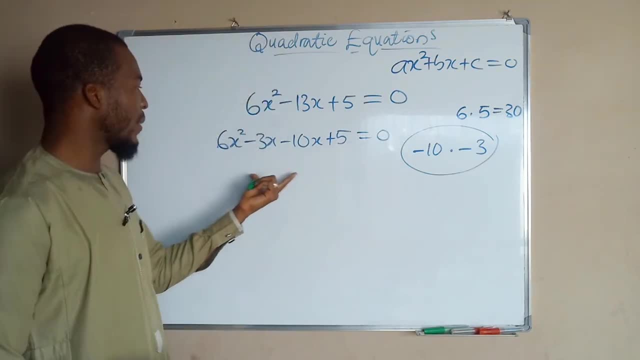 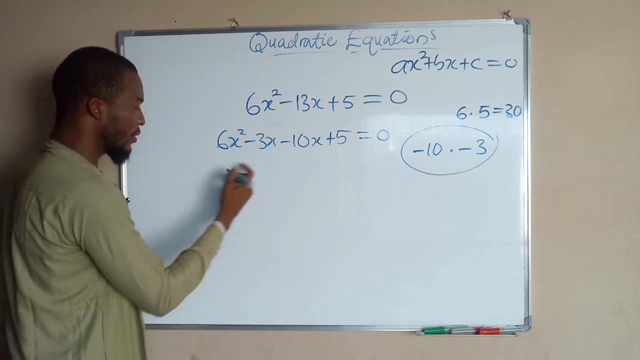 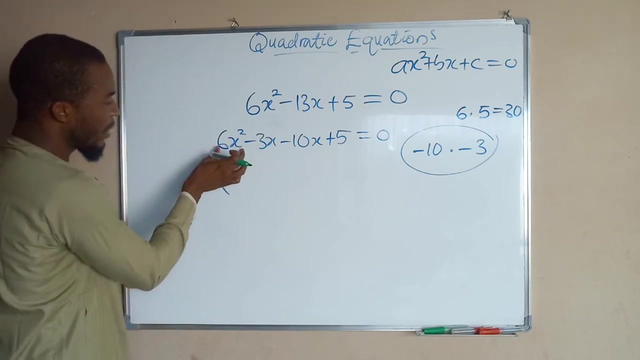 This is equal to 0. Then we are going to factorize in batches, the first two and the second two. The first two among numbers: they have 3 in common, so we have 3.. Among the unknown variables, we have x in common From the first term. if you divide this by this, you are going to 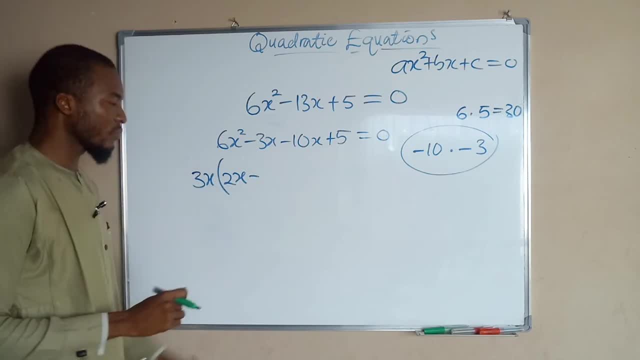 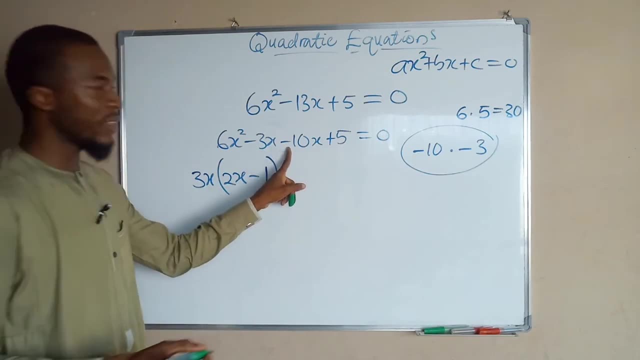 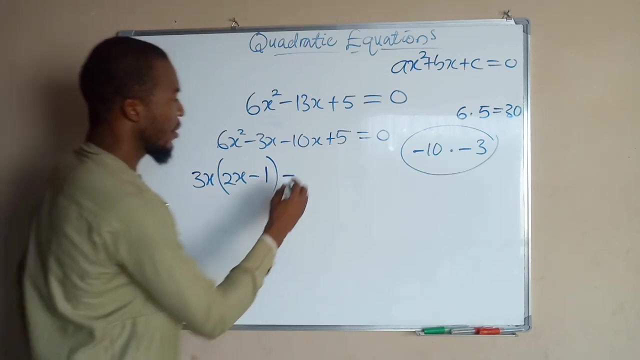 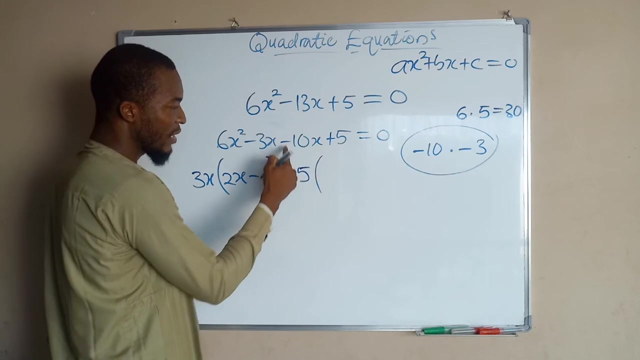 obtain 2x minus. Already we have factor 3x out, so we are left with only one here. Then you drop your sign, which is minus. Among these two terms we have 5 in common, so we have 5.. Then in the bracket, if you divide negative 10x. 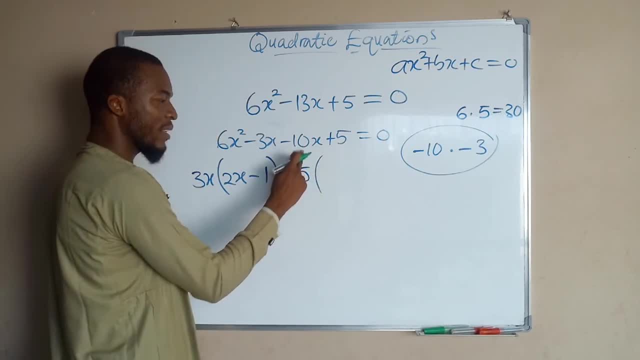 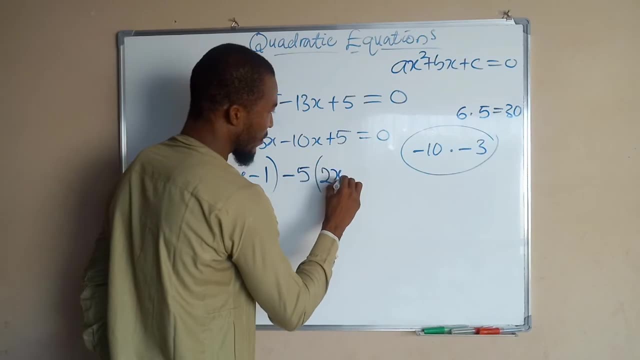 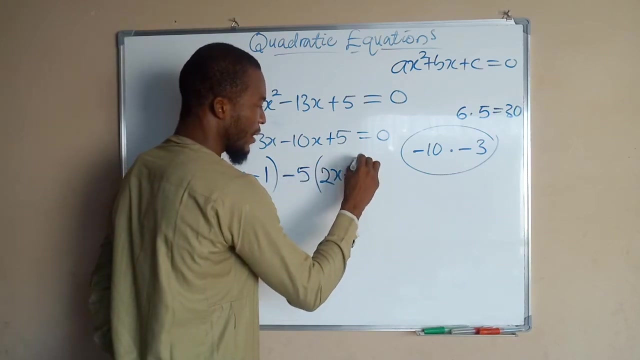 Cancel negative having positive sign. Then 10 divided by 5, we have 2.. Then x has no x to divide, so we have x. Then 5 divided by negative, 5 is going to make it negative 1. The whole of this equal to 0.. 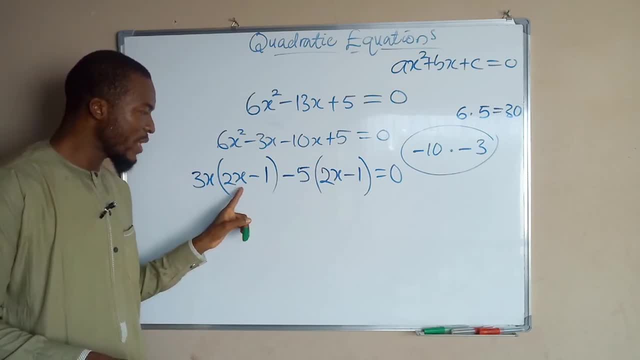 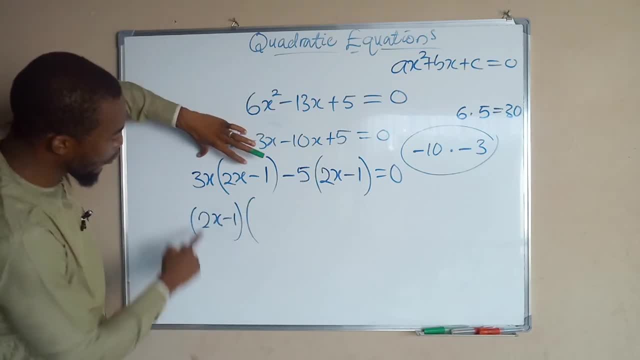 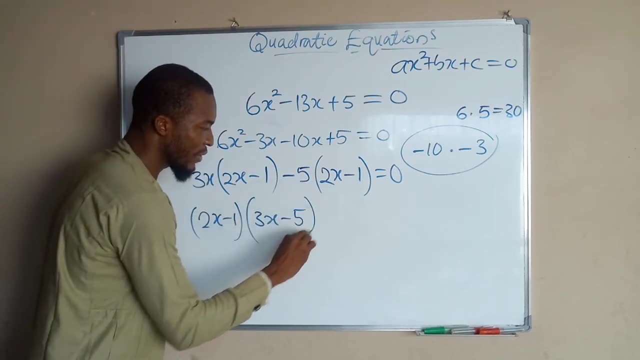 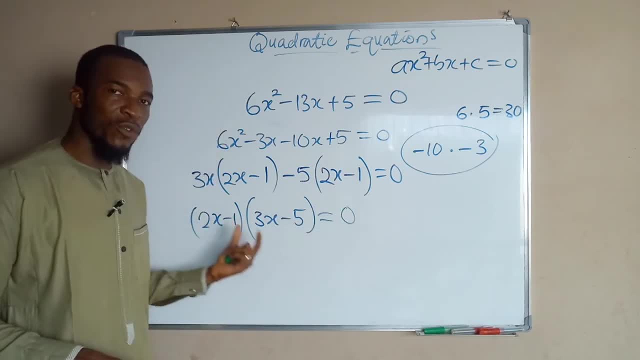 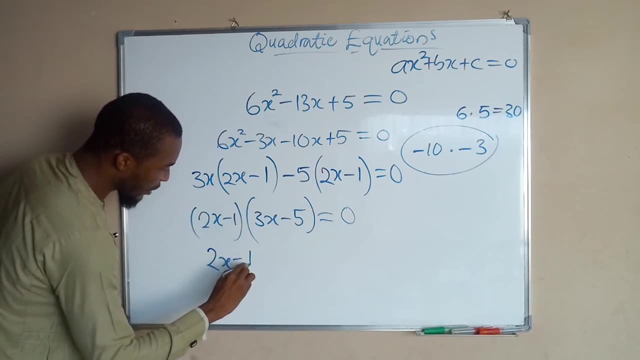 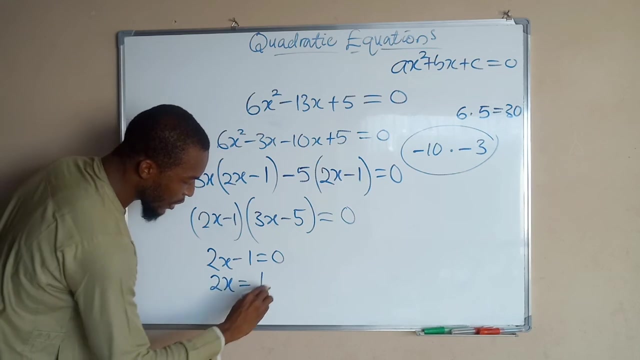 And all of this equal to 0.. Now we have our two factors which we are going to set each to be equal to 0. If you set the first one, 2x minus 1, to be equal to 0. If 1 crosses equality sign, it becomes 2x equal to positive 1.. 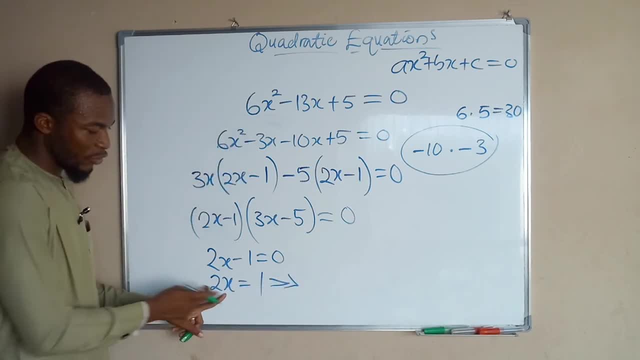 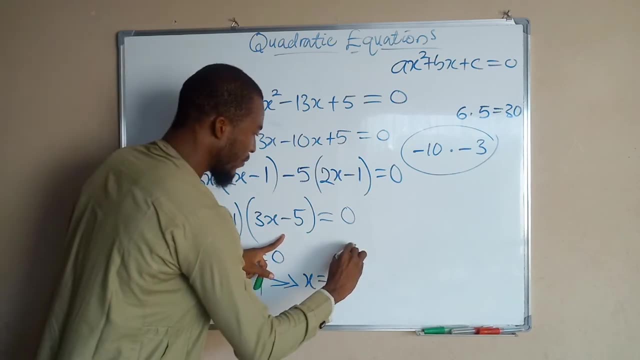 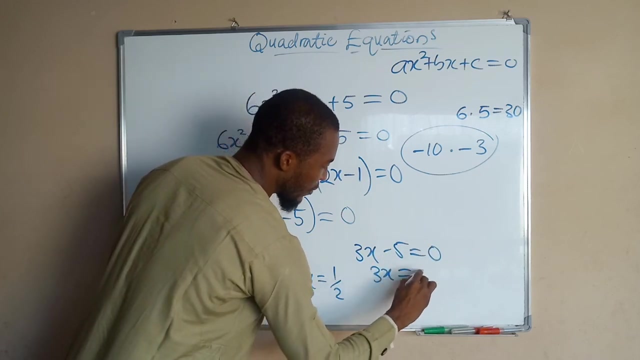 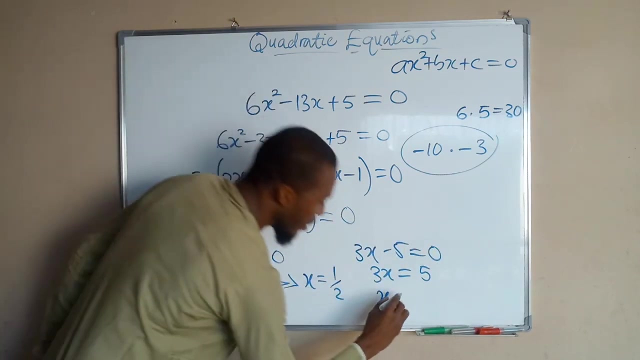 that x equal to 1 divided by 2. so x equal to 1 over 2. then from the second factor we have 3x minus 5 equals to 0. 3x will be equal to positive 5 if negative 5 crosses over. and to find x we are going to divide both sides by 3 and x. 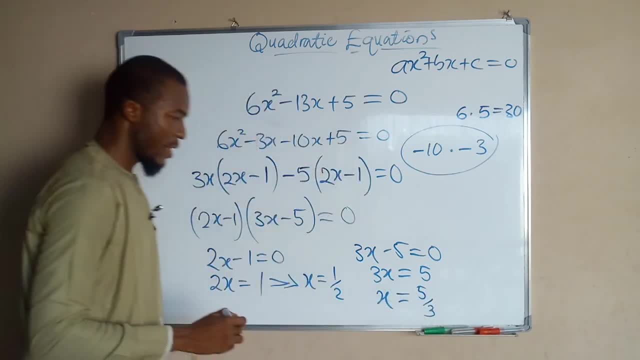 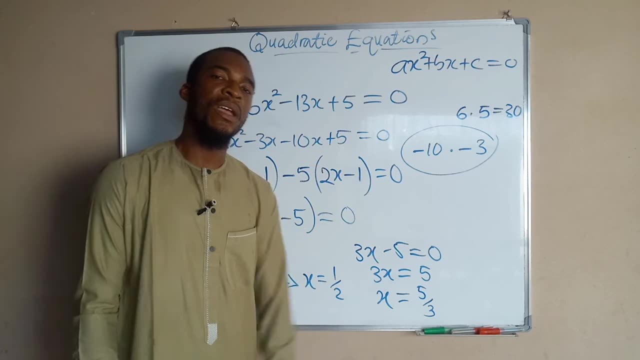 now equals to 5 over 3. hence, the root of this quadratic equation are 1 over 2 and 5 over 3, and this is all I have for you today. thank you for watching and do have a nice day. 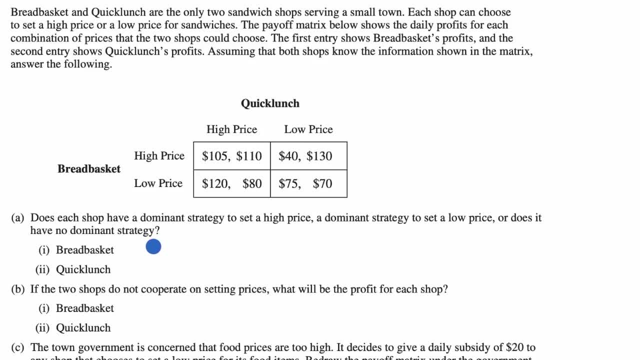 What we have here is a free response question that you might see on an AP microeconomics type exam that deals with game theory, And it tells us bread basket and quick lunch are the only two sandwich shops serving a small town. So we're in an oligopoly situation. 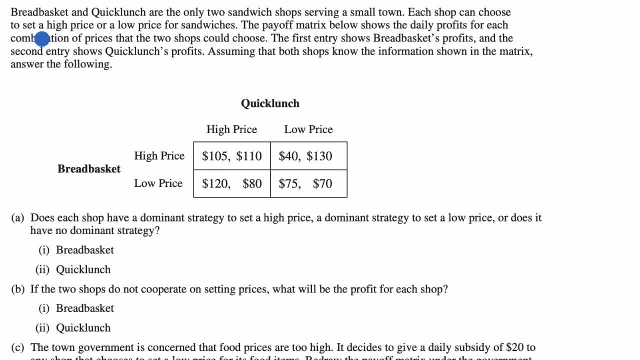 where we only have a few firms. Each shop can choose to set a high price or a low price for sandwiches. The payoff matrix below shows the daily profits for each combination of prices that the two shops could choose. The first entry shows bread basket's profits. 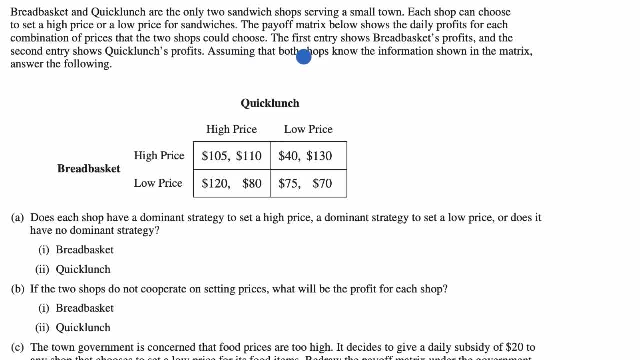 and the second entry shows quick lunch's profits. Assuming that both shops know the information shown in the matrix, answer the following. So just to make sure I understand what's going on here. this is saying that, for example, if bread basket can either choose: 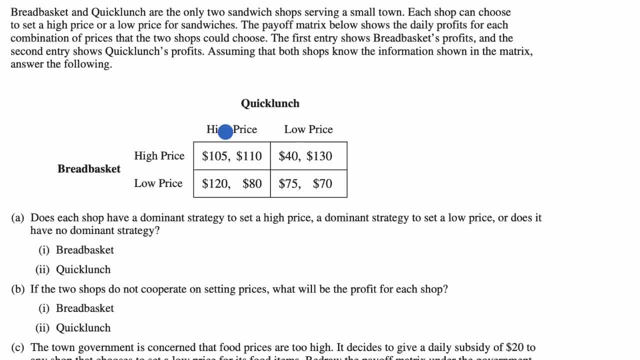 to charge high prices or low prices. quick lunch can either choose to charge high prices or low prices. If bread basket chooses high prices and quick lunch also chooses to charge high prices or low prices, then what this tells us is the first one is: bread basket's profit per day would be $105,.